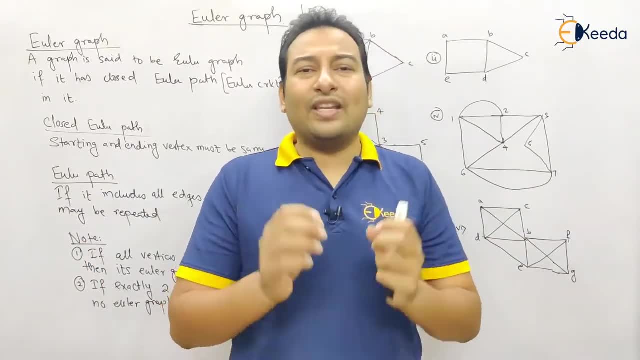 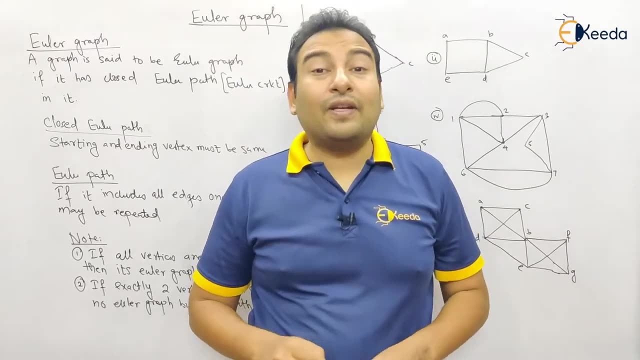 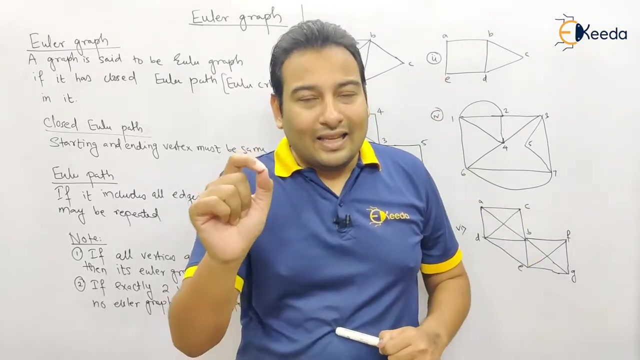 this type, this topic, so very important topic and it's very simple topic. so let us start with the definition. first of all, a graph is said to be Euler graph if it contains closed Euler path. first point clear. what is the point? a graph is Euler graph if it contains closed Euler path, or closed Euler path is also called. 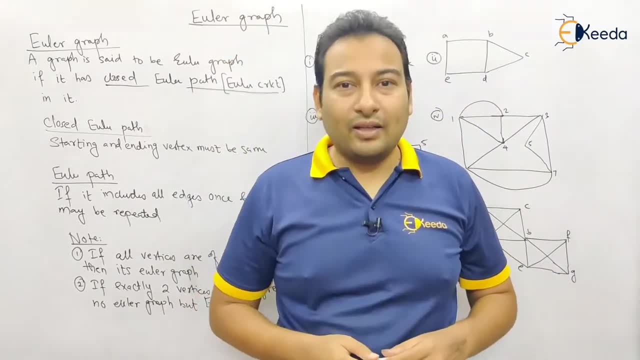 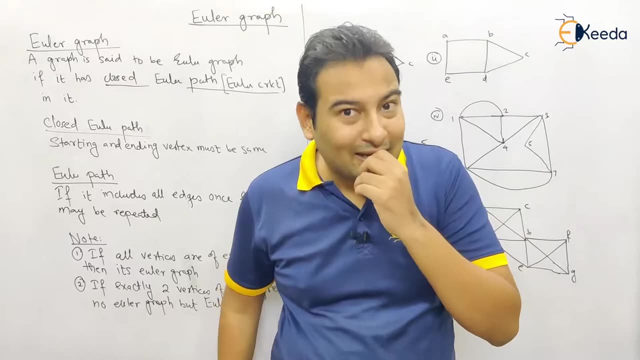 Euler circuit. so what do you mean by closed Euler path? closed mean the starting and ending of a closed Euler path must be same, like open walk, close walk that we discussed in the last video. same story: if the starting and ending vertex is same, then it is called a closed Euler. 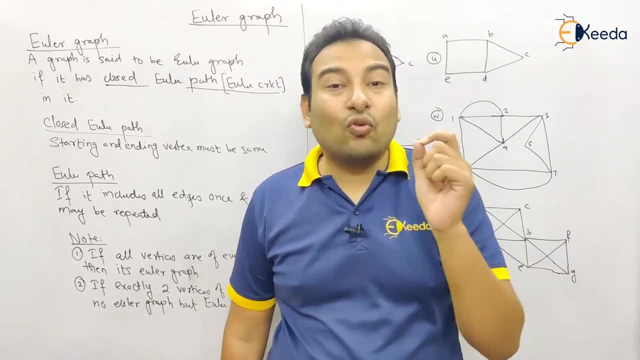 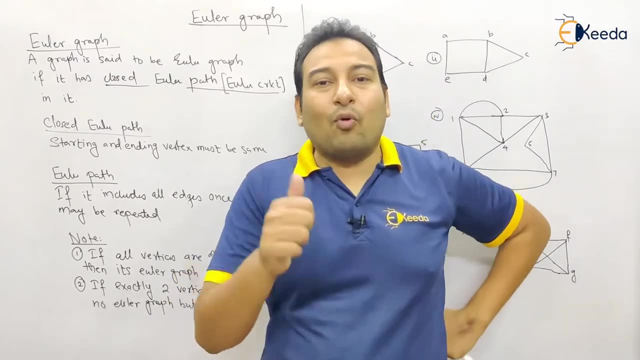 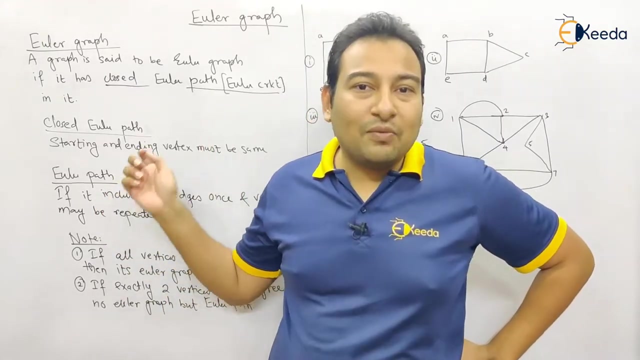 path. so a graph is Euler graph if it has closed Euler path. that means the starting and ending vertex is same. so we got it. what is a Euler graph now? the point is, what is Euler path? Euler path means each and every vertex must be visited once and there is no change in Euler path. 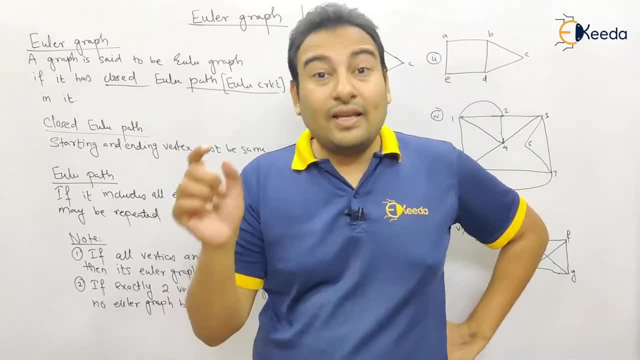 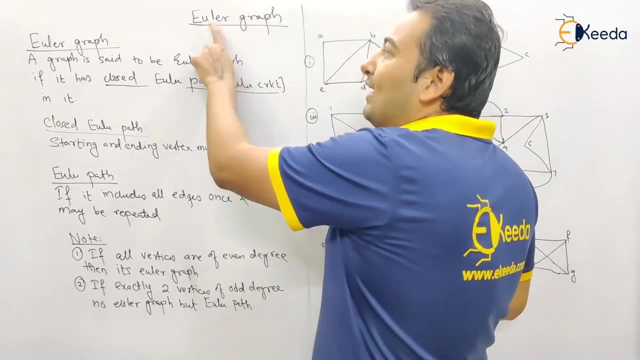 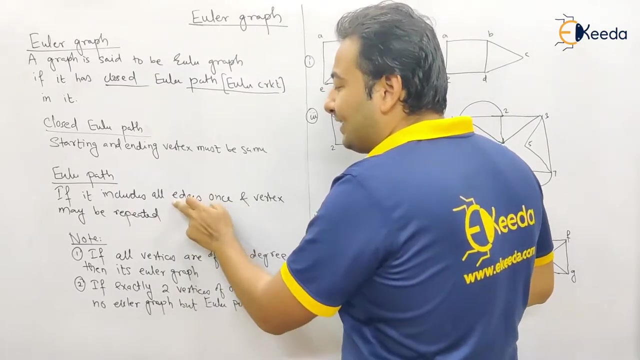 so this is Euler path and there is no restriction on sorry. each and every edge must be visited once and there is no restriction on vertices. see how I remember this: Euler E, ages E, so it includes all the edges ones, edges E and Euler E, it includes all the edges, ones and vertex may be repeated. so this is. 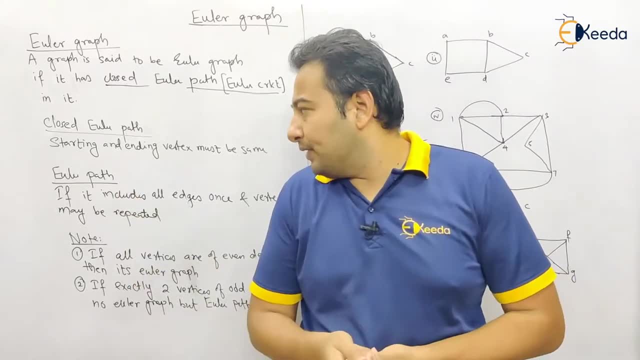 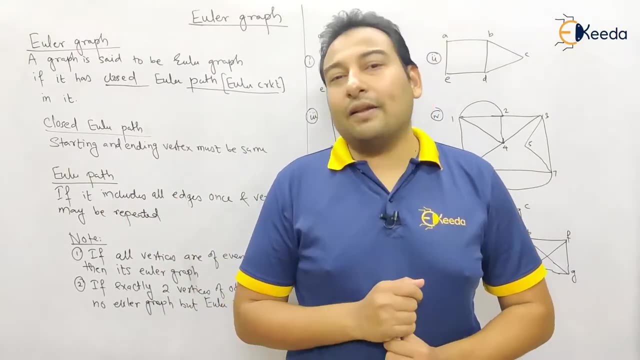 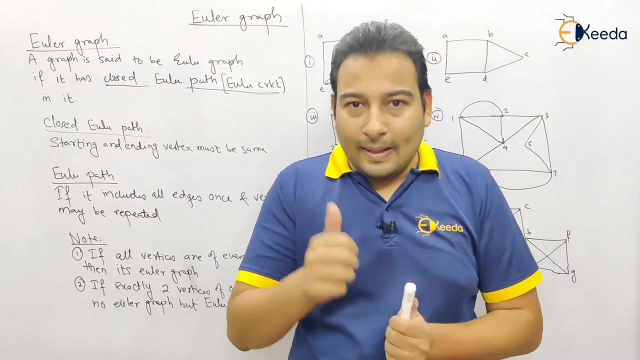 your Euler path. now you might be thinking: is it similar to walk or a? is there any difference between walk and a Euler path? yes, there is a difference and the difference is: first of all, let us check what is the similarity- similarity between walk and Euler path. both the method says edge should not be. 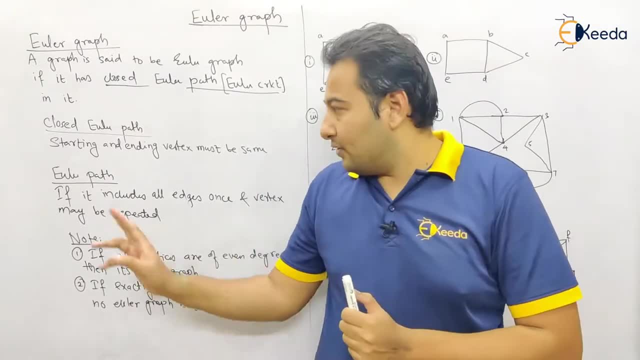 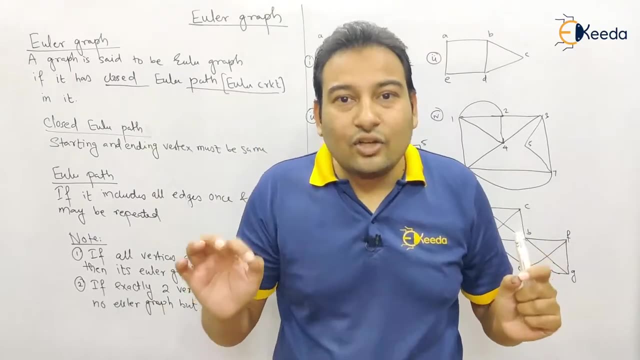 visited more than once, and there is no restriction on vertices. so here also the same condition. there also it is the same condition, but in case of walk it was not necessary to visit each and every edge, but in case of Euler path it is necessary to visit each and every edge. 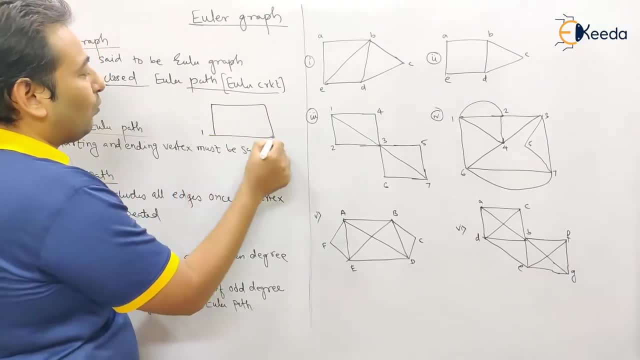 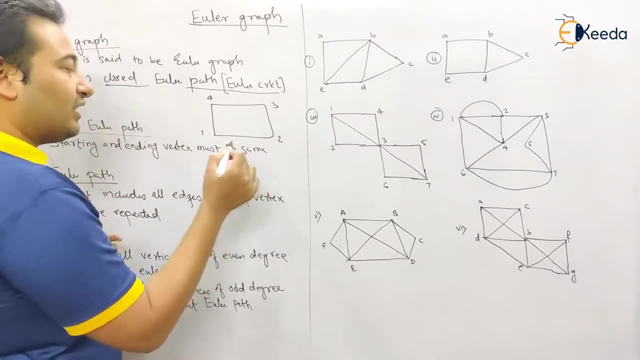 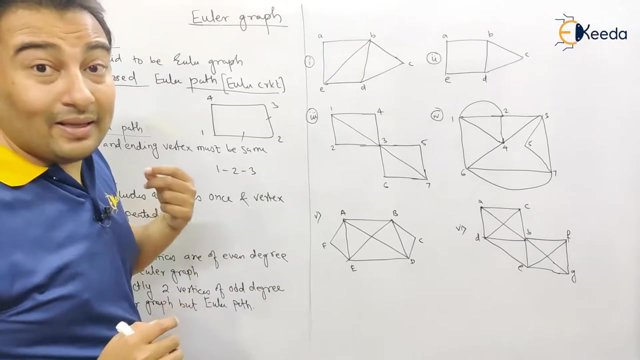 so let me give an example. suppose this is the graph one, two, three, four. so if I talk about walk one, two, three, it's a walk. see here: one, two and three. this is visited once. no restriction on what I said. it's a walk, but it's not a Euler. 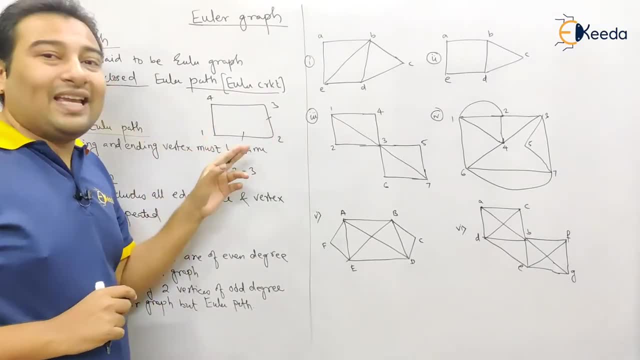 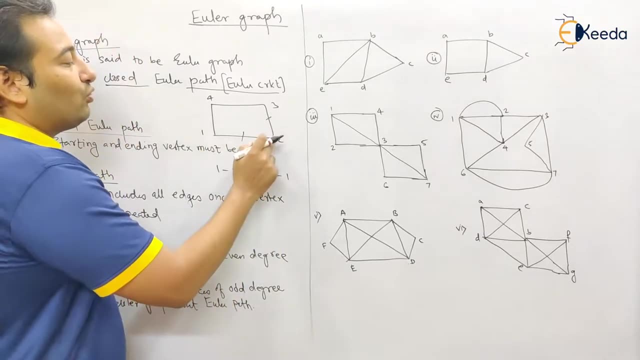 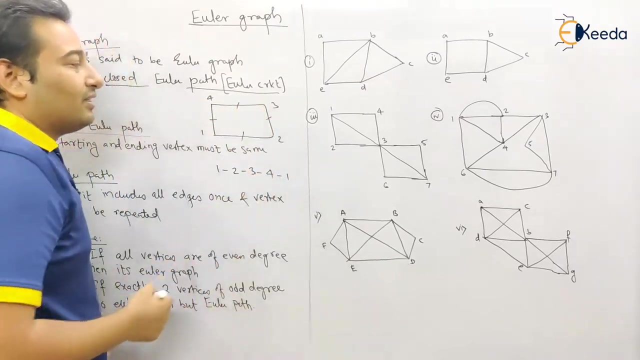 path. why? because in case of Euler path, every edge must be visited. these two edges must be visited. if you extend this, see here: one, two, two, two, two, three, three, two, four and four to one. now you can see: all the edges are visited once, then it is called Euler path. 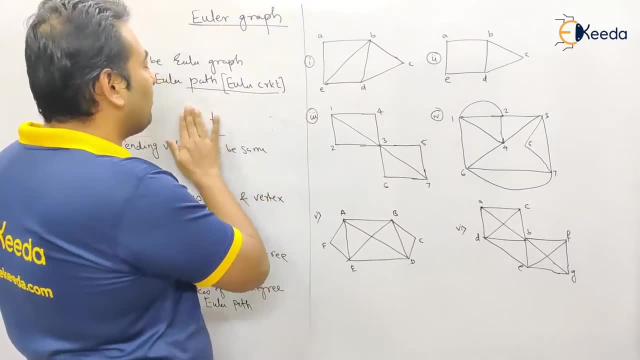 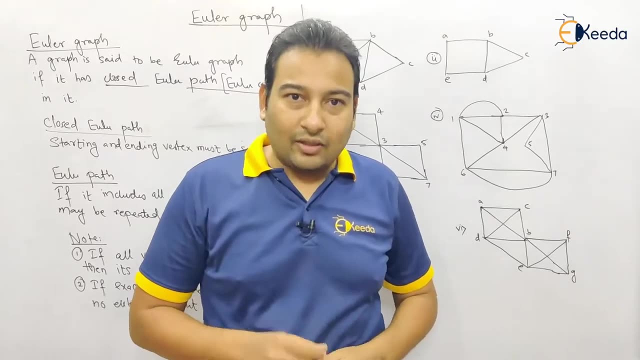 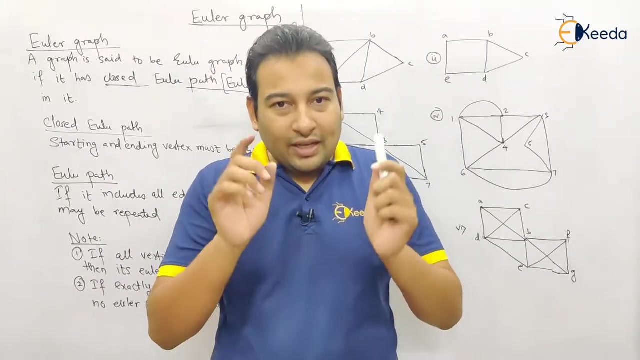 is this concept clear Euler path and what is the difference between walk and Euler path? so let me repeat again. first of all, what is a Euler graph? it contains closed Euler path. closed Euler path means what starting and ending vertex should be same. what is the Euler path and what is the difference between walk and Euler path? 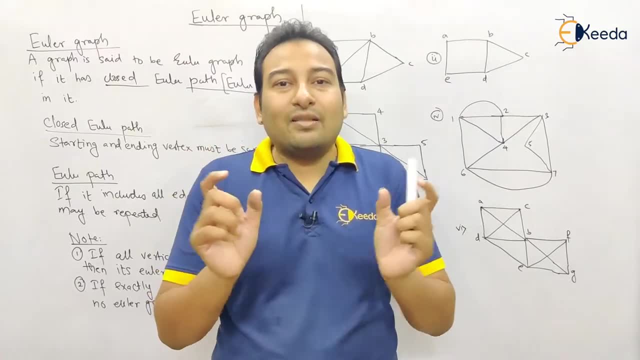 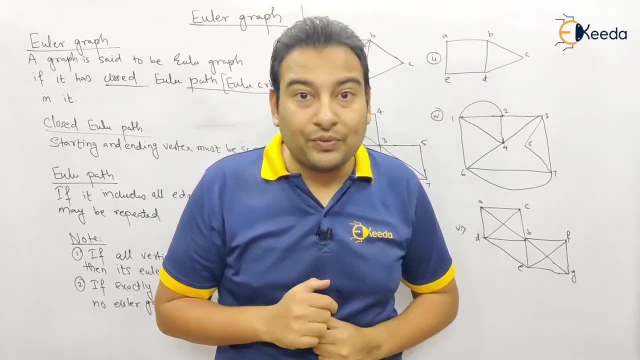 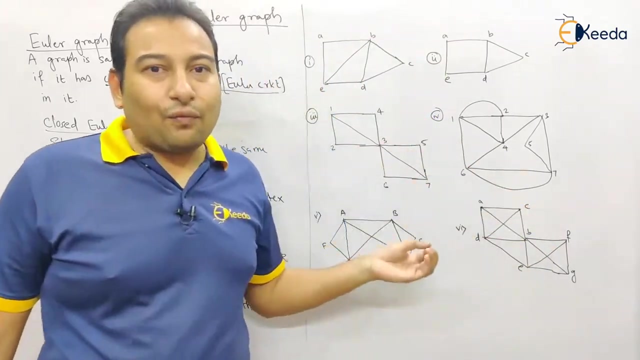 in both edges must not be visited more than once. no restriction of what I says. but in case of Euler path, all the edges must be visited. but that was not the condition with the walk. now there are few graphs given in front of us and we need to check whether they are Euler graph or not first of all. if you 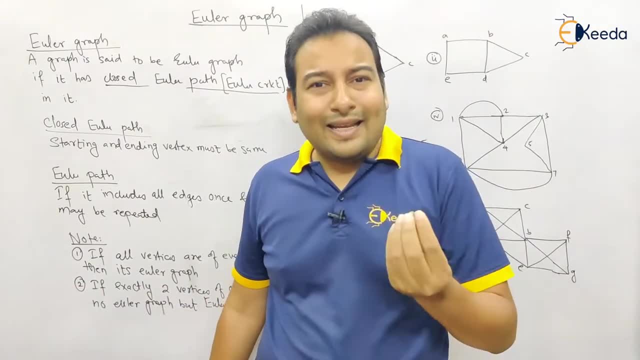 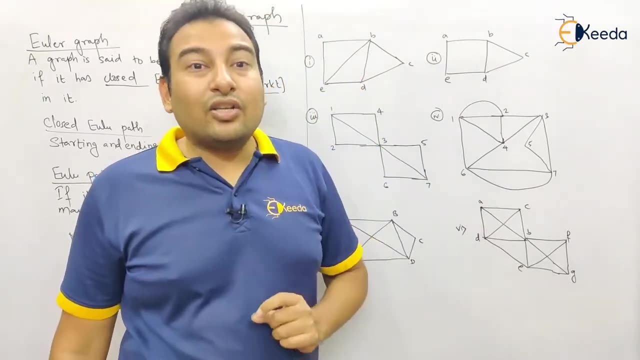 remember point number one, very important point in get exam, MCQ exam or any completed exam, by looking at the graph BTOB model of itsет, you can see whether it is a Euler graph or not And the condition is in case of Euler graph: 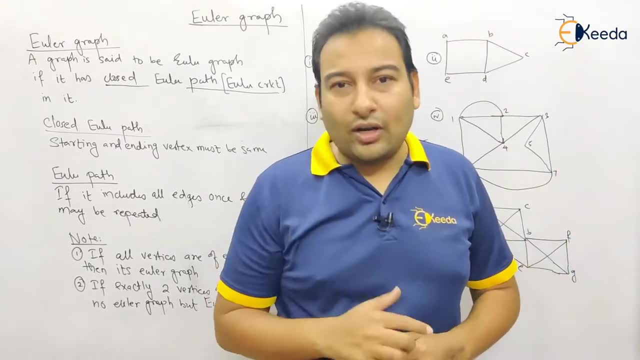 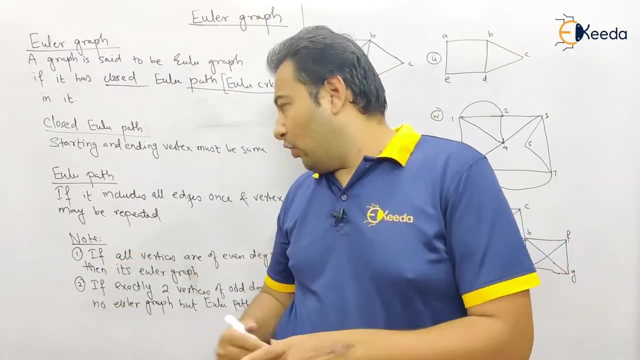 all the vertices have even degree. So first point, very important point, If a graph is Euler graph, then all the vertices are of even degree. So this is the first point, very important point. So all the vertex should be of even degree. 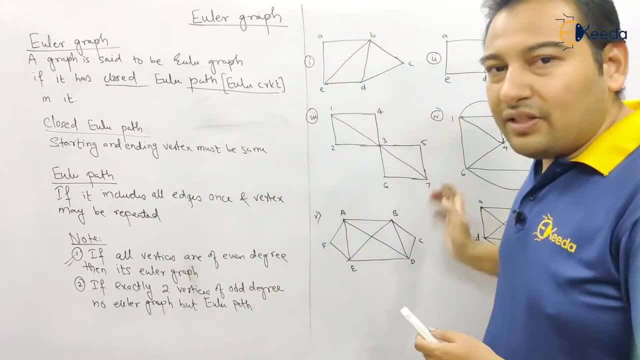 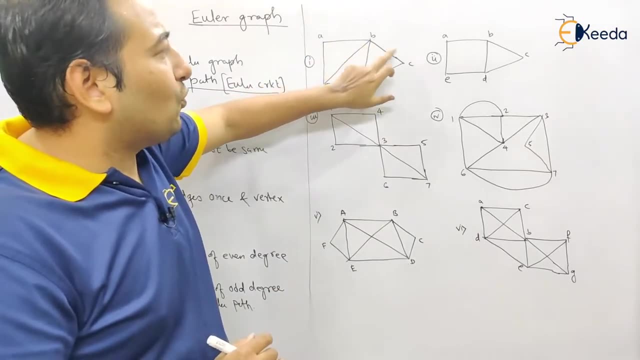 then the graph is said to be Euler graph. So let us check which graph is a Euler graph or not. All the vertices should have even degree. see here: Two its degree is four. Two its degree is three. Is it a Euler graph? 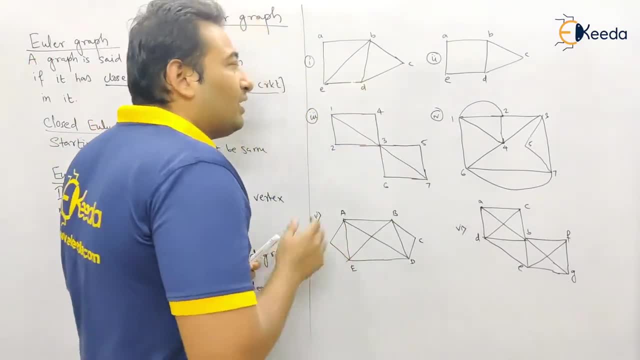 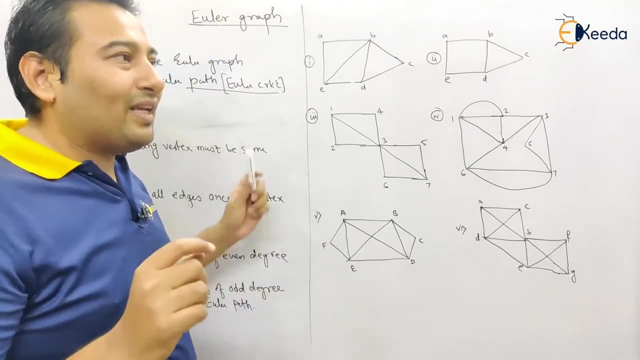 No, because this particular vertex has odd degree. Therefore it's not a Euler graph. So the condition for Euler graph is: all the vertices should have even degree. There is one more point. see, There is one more point. We'll discuss all the graph, don't worry. 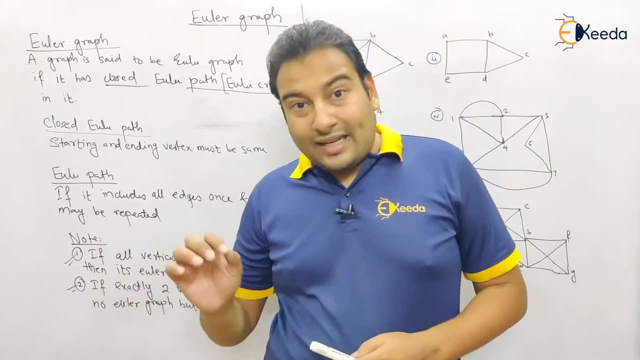 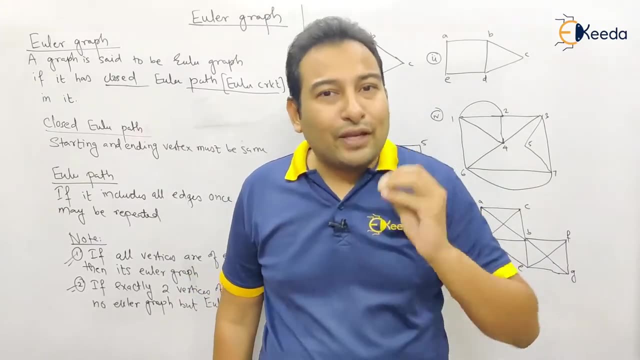 First of all, let us understand. There is one more point: If there is a vertex with odd degree, it cannot be Euler graph, Because what is the condition for Euler graph? All the vertices must have even degree. If there is a vertex with odd degree, 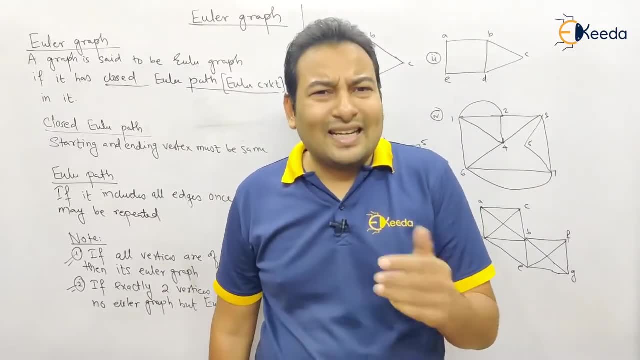 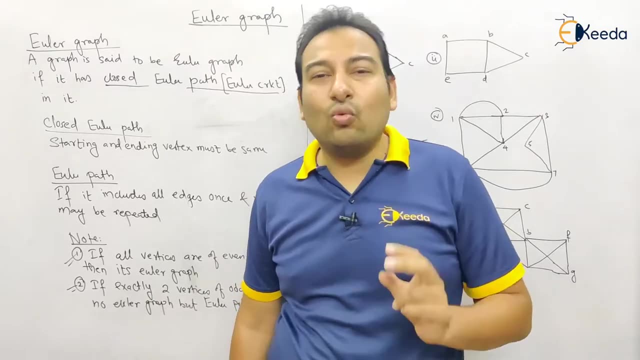 it's not a Euler graph. Now there is one more condition. It's an additional condition: If there are exactly two vertices with odd degrees. if there are exactly two vertices with odd degrees, obviously it can't be Euler graph, Because if there is at least one vertex of odd degree, 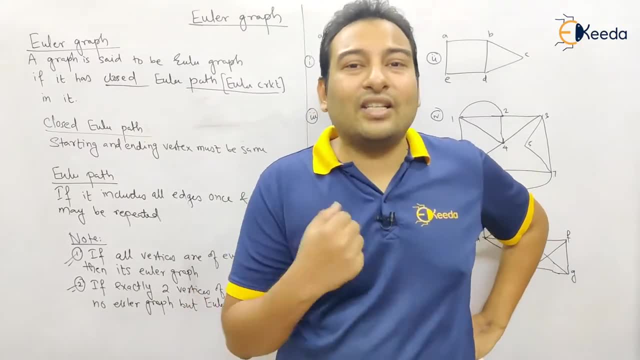 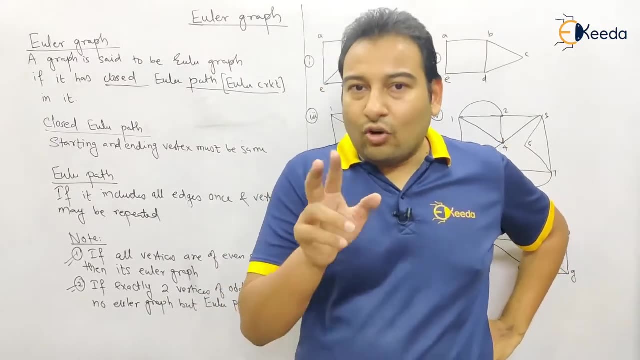 it cannot be Euler graph. Now we are talking: if there are two vertices with odd degrees, obviously it can't be Euler graph. there can be a Euler path. What is the difference between Euler graph and Euler path? Euler graph contains closed Euler path. 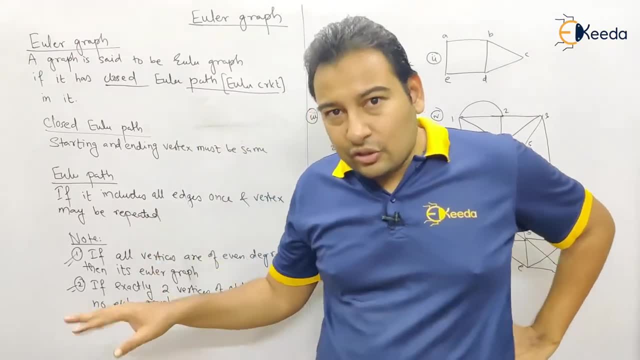 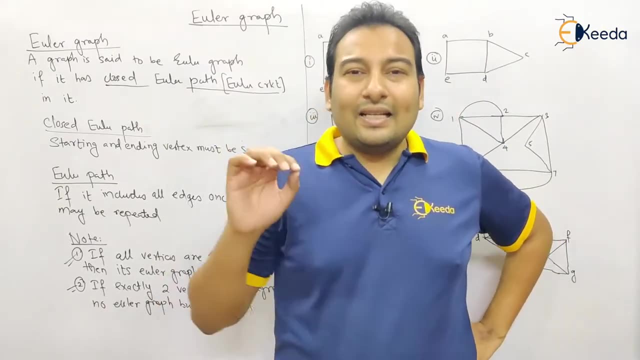 And what is closed Euler path? Starting and ending vertex is same. So if there are vertices with exactly two vertices with odd degree, there cannot be Euler graph. That means there cannot be closed Euler path. That means starting and ending vertex is not same. 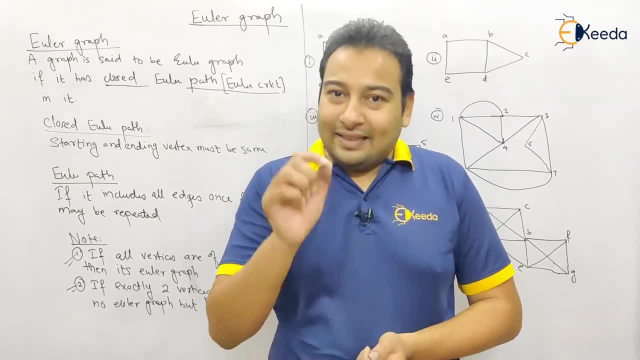 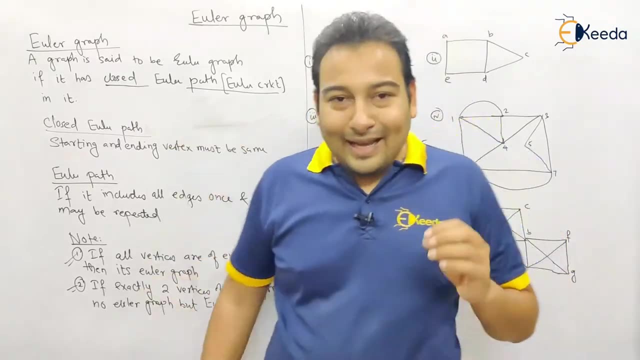 but there will be a Euler path. That will see, there will be a Euler path, Start from one vertex with odd degree and that will end at the other vertex of odd degree. So this is the entire discussion. I hope this is clear. 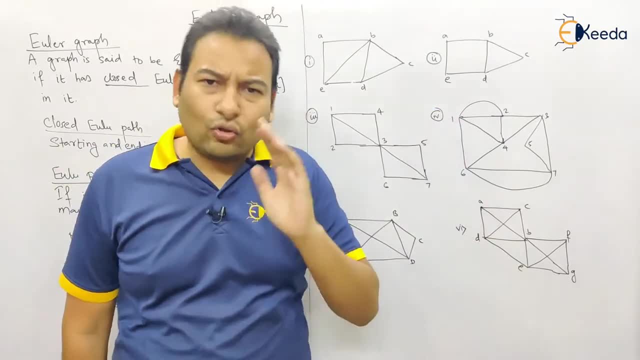 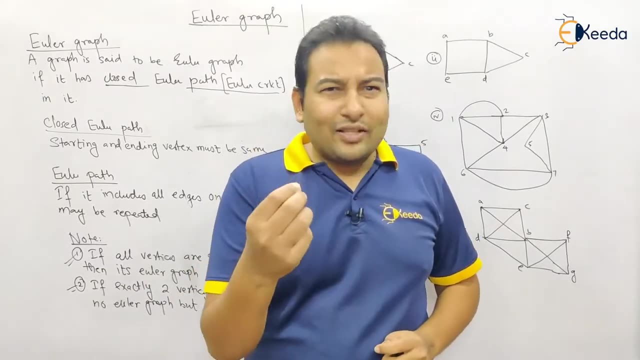 If not, don't worry. While if we see this example, the topic will be very clear to you. So let me repeat again: See, it's a bit, you can say, complicated to understand, But once you understood, it's the simplest topic. 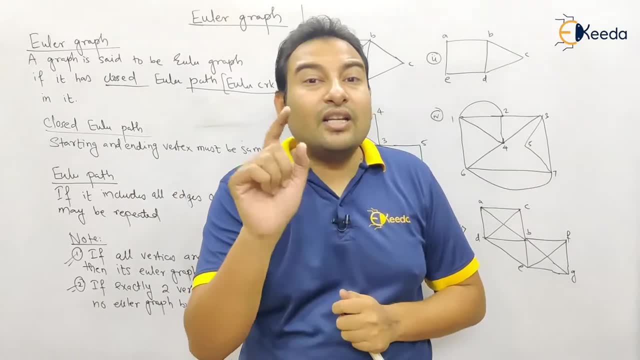 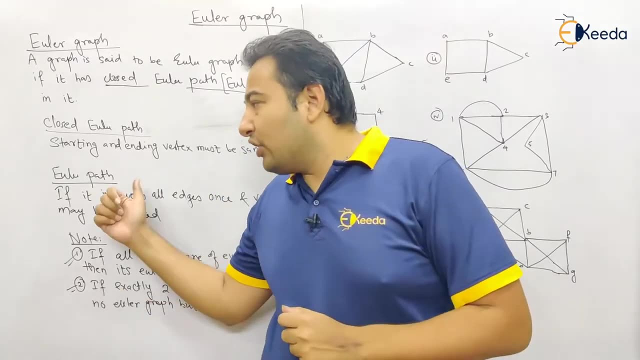 So let us start again. What is Euler graph? It must contains closed Euler path. Closed Euler path is what Euler circuit? That means starting and ending vertex should be same. So what is Euler path? All the edges must be visited once. 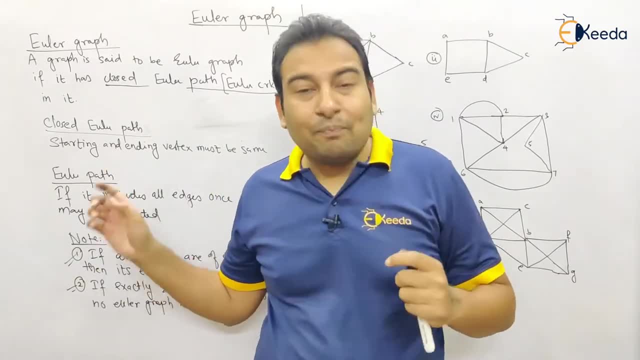 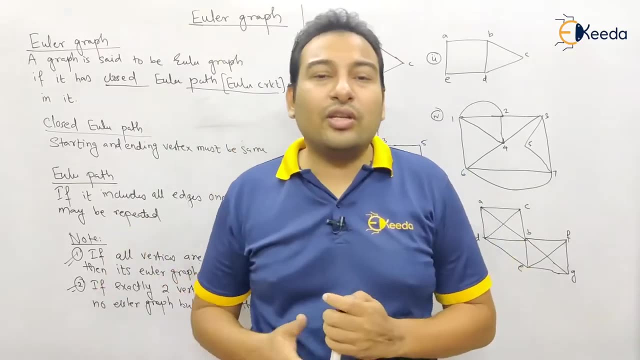 There is no restriction on vertices. What is the difference between walk and path, Walk and Euler path? In case of walk, no condition that all the edges must be traversed. But here, in Euler path, the condition is all the edges must be traversed once. 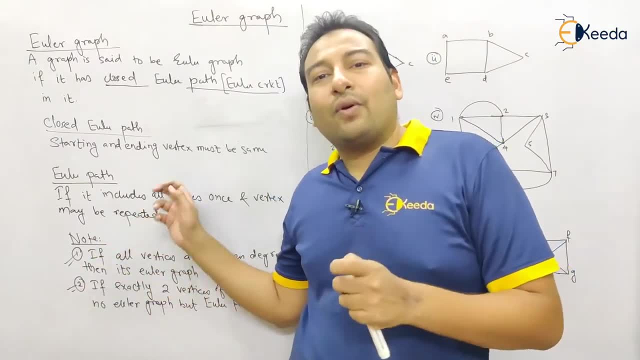 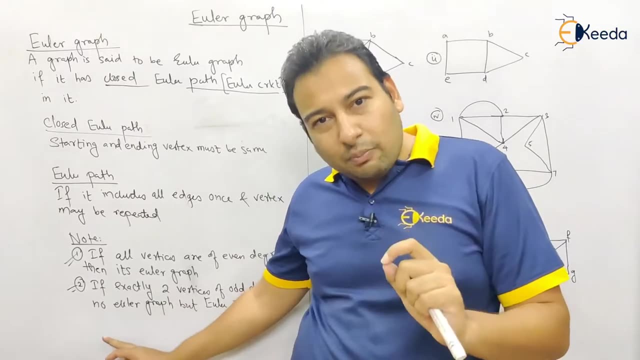 How to check whether a graph is Euler graph or not. If all the vertices have even degree, then it is a Euler graph. If there is at least one vertex with odd degree, it's not a Euler graph. There is a special case you can say. 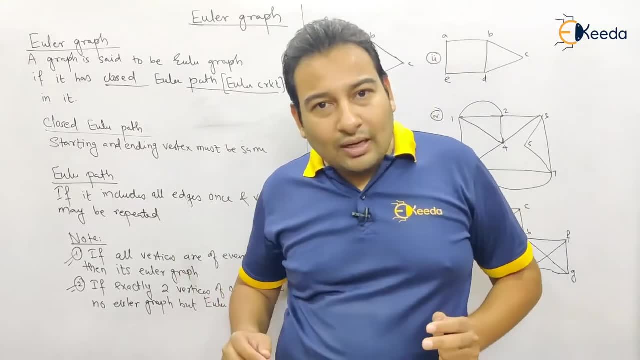 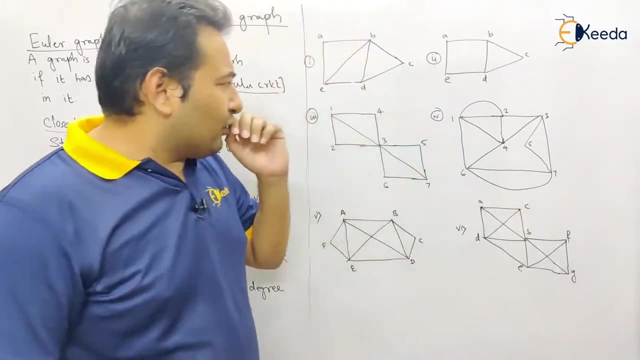 Exactly two vertices with odd degree. obviously it cannot be Euler graph, but it will be Euler path, which will start from one vertex of odd degree and it will end at the other vertex of odd degree. So no problem, don't worry. whatever we discussed, 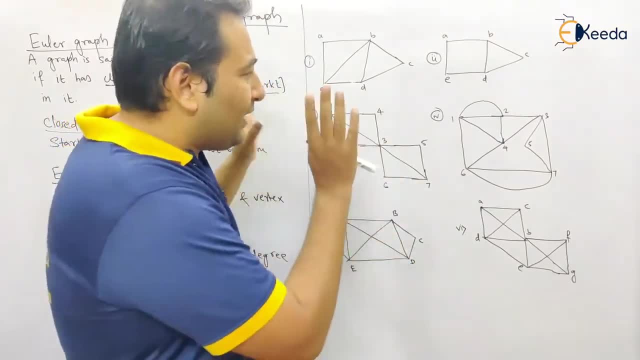 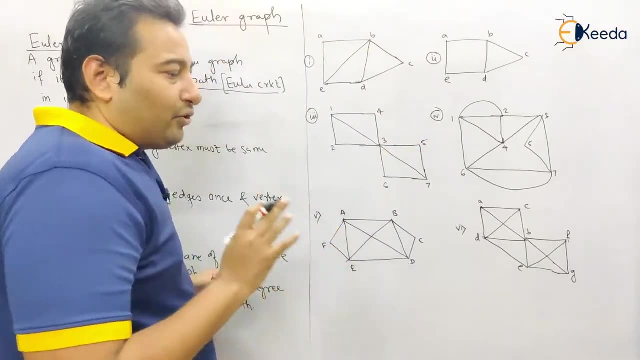 If you didn't understand anything, no problem, Let us understand with the help of example, and it will be very clear. Let us start First of all. my aim is to check whether the graphs are Euler graph or not. If it is a Euler graph, 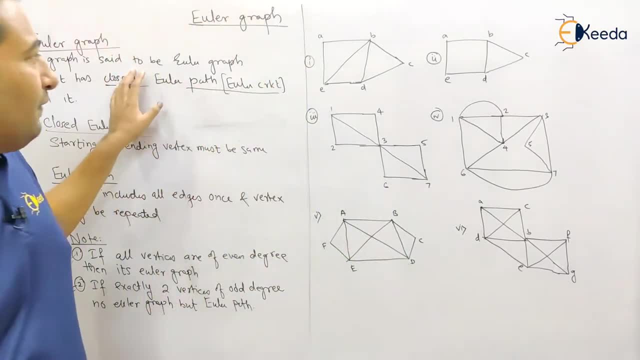 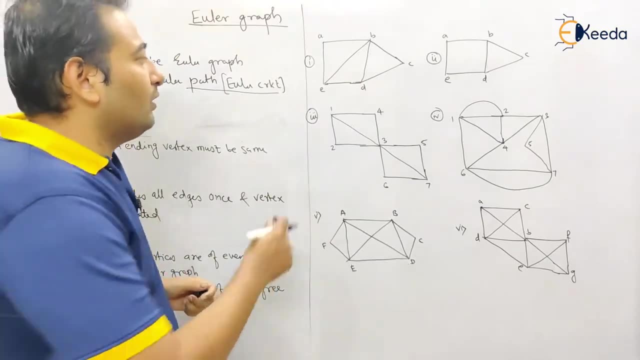 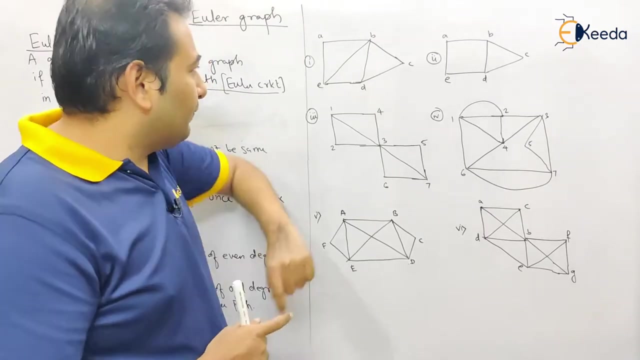 so obviously there will be Euler circuit. If it is a Euler graph, there will be a Euler circuit or closed Euler path, So that we need to write it down. So let us discuss the first one. What is the criteria for checking? All the vertices must have even degree. 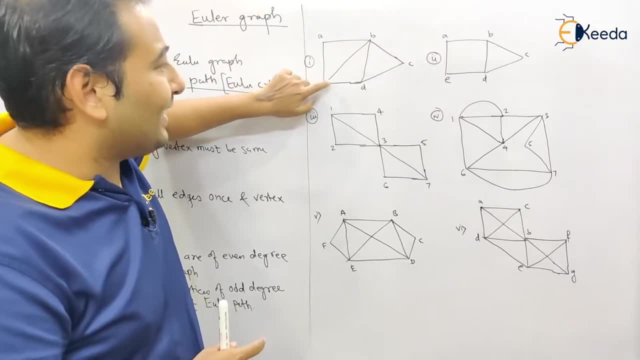 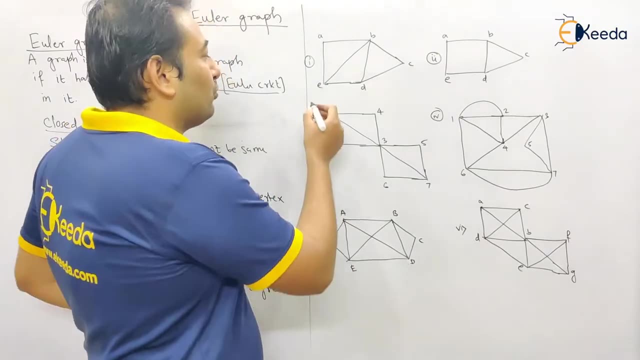 See, the degree is 2, even 1,, 2,, 3, the degree is odd. Story over: There is a vertex with the degree odd. It is not a Euler graph, So not Euler graph. First point is clear. 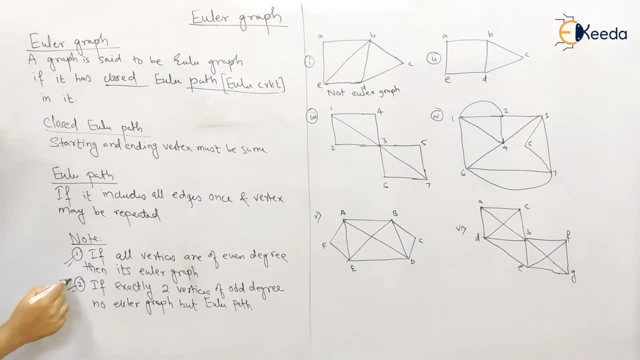 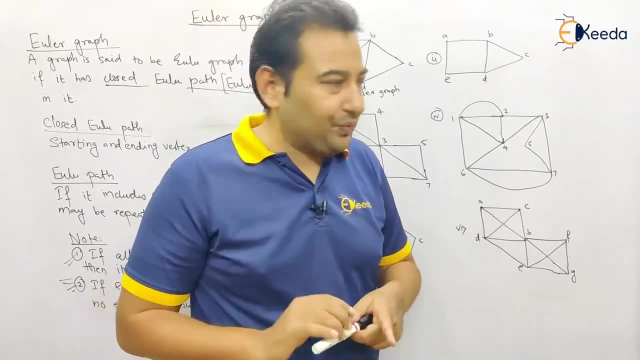 Now we need to check for a special case, And this is the special case: If there are exactly two vertices with odd degree, there can be a Euler path. So let me check. This is degree 2.. This is degree 4.. 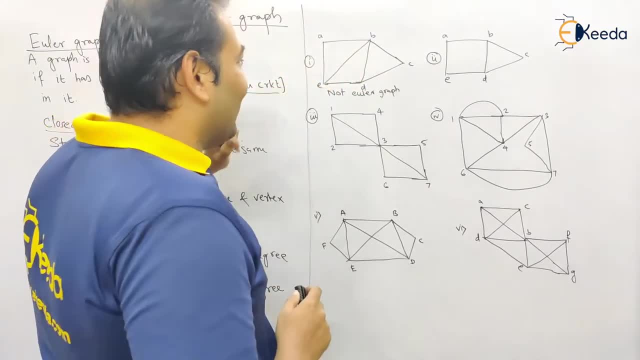 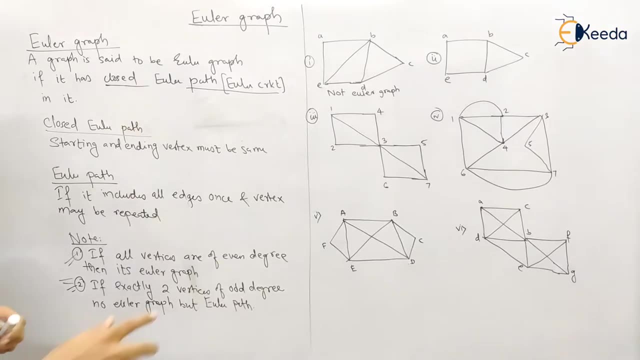 This is degree 2.. This is degree 3.. And this is degree 3.. That means in graph number 1, that means in graph number 1, there are exactly two vertices. There are exactly two vertices with odd degree. See at least one vertex with the odd degree. 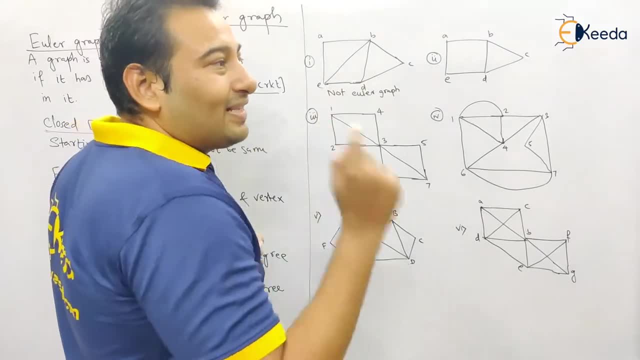 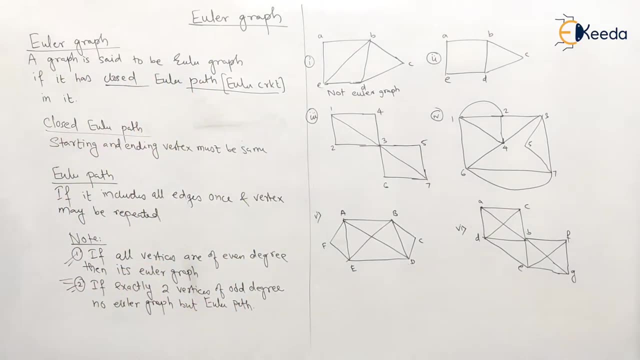 it cannot be Euler graph. That story is over. But if there are exactly two vertices with odd degree, there will be a Euler path And that will start from. that will start from- let me extend this point- that will start from one vertex of odd degree. 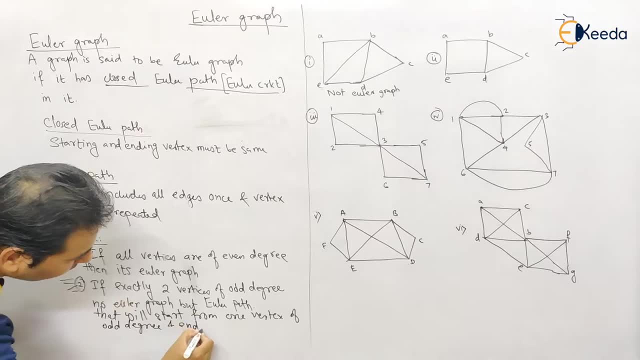 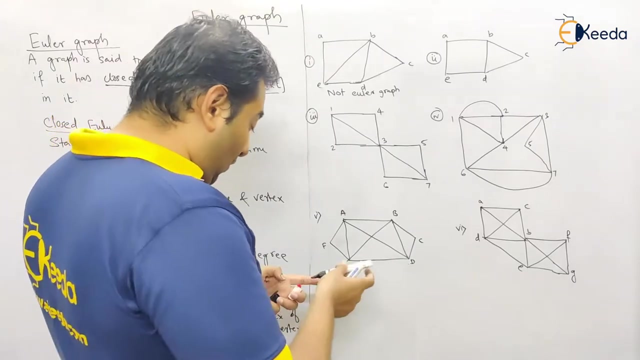 and end with other vertex of with odd degree. So not a Euler graph because there are two vertices with odd degree. There will be Euler path that will start from one vertex of odd degree and end with the other vertex with the odd degree. So this is one vertex with the odd degree. 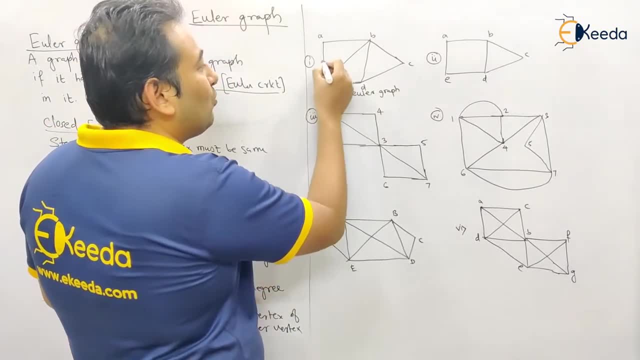 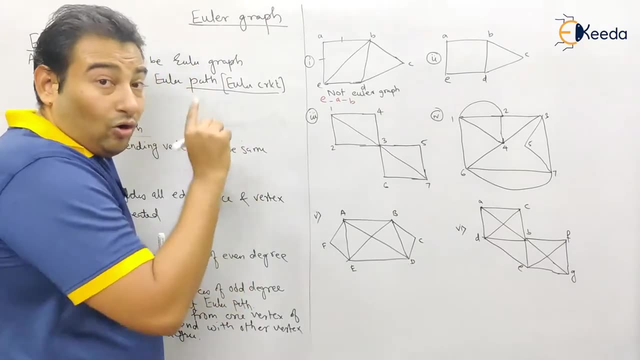 So let us start with E. So the path will be from E to you can go to A, From A to B. what is the condition? Edges must be visited once only, and all the edges must be covered. So from B you can come to E. 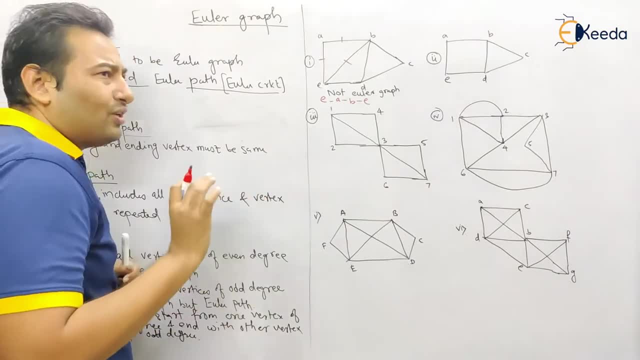 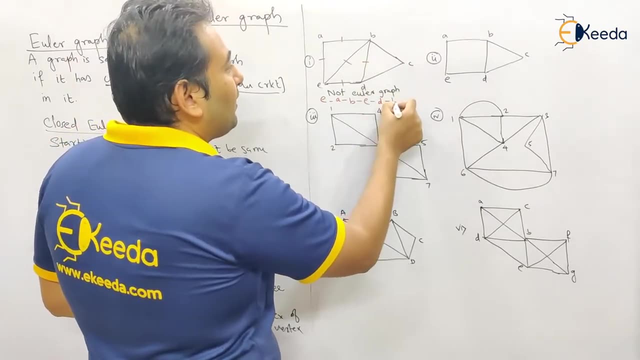 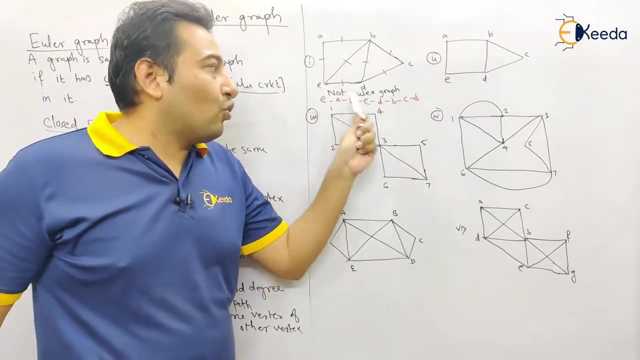 So there is no problem. E is repeated, so that is perfectly fine, because there is no restriction on edges, vertices. Then it will be D, then it will be B, then it will be C and D. See, here it is called a Euler path. 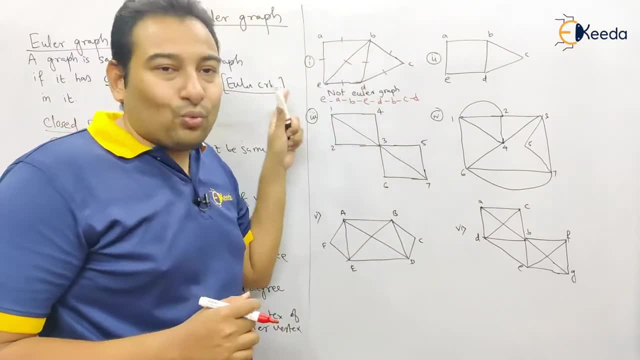 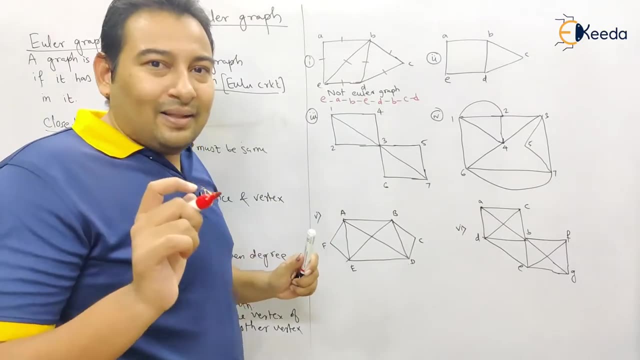 Why it is called Euler path. See, all the edges are traversed once. There is no edge which is left, and it is traversed once, No restriction on vertices, and therefore it is a Euler path. Suppose the starting and ending point is same. 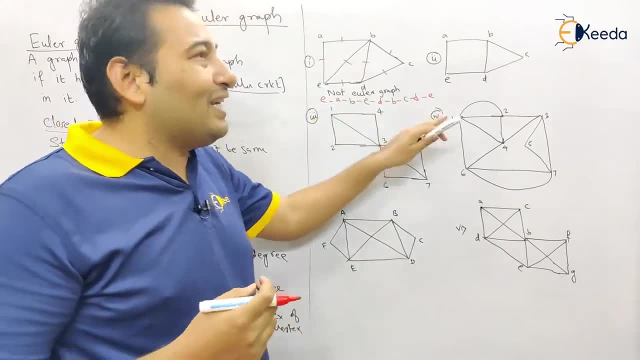 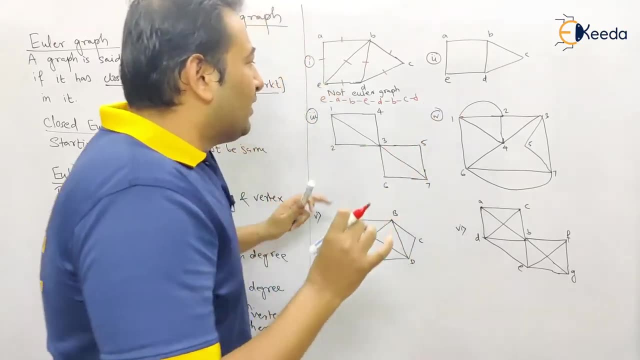 Suppose I am giving the example, Suppose the starting and ending point is same, then it is called closed Euler path and then that becomes a Euler graph. But here obviously it is not a Euler graph that we know. That means there is no closed Euler path. 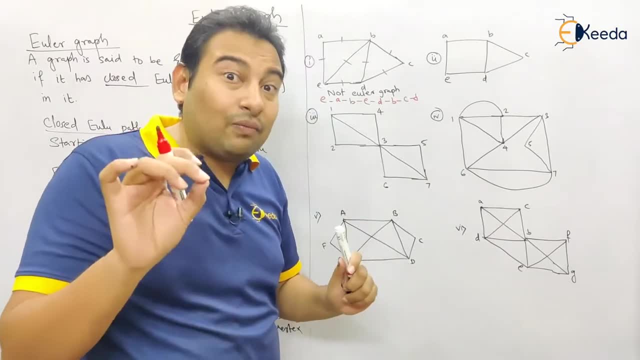 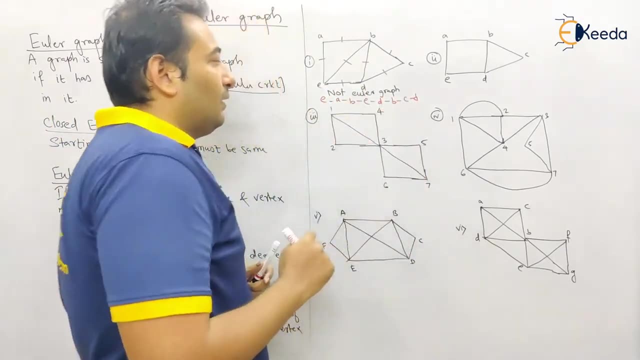 but there is a Euler path- Not closed, but there is a Euler path that will start with one vertex of odd degree and end with the other vertex of odd degree. Now you can start from D also and you can come back to E, So make sure that exactly two vertices of odd degree. 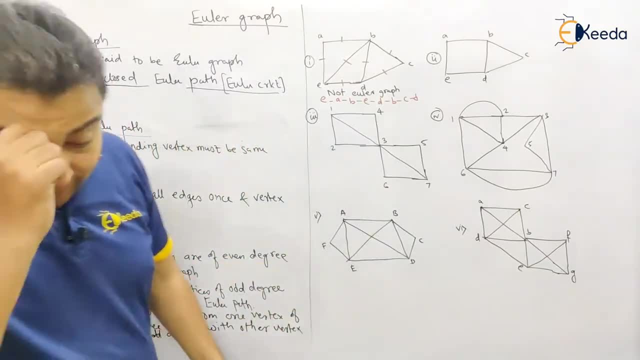 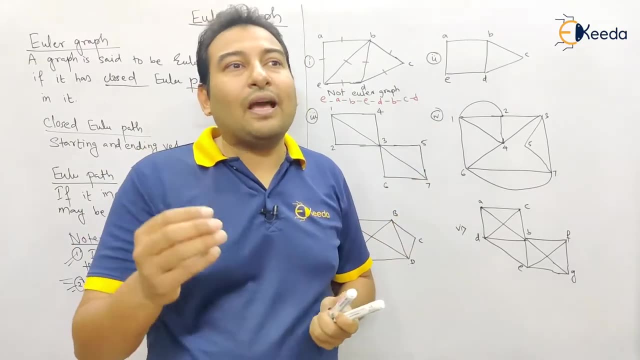 start from one and end at the other. Let us move on Now. the question is: what if, see this is the example in which we have two vertices with the odd degree, What if we have three vertices with odd degree? Please tell me the answer. 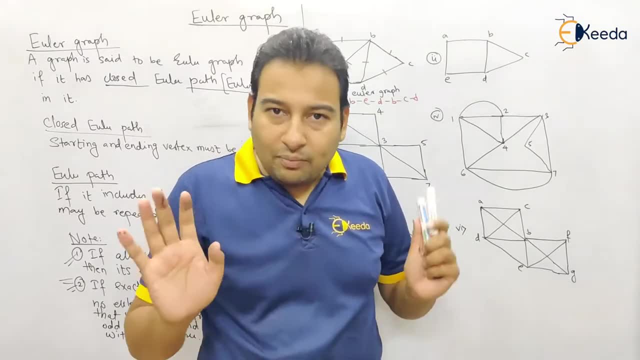 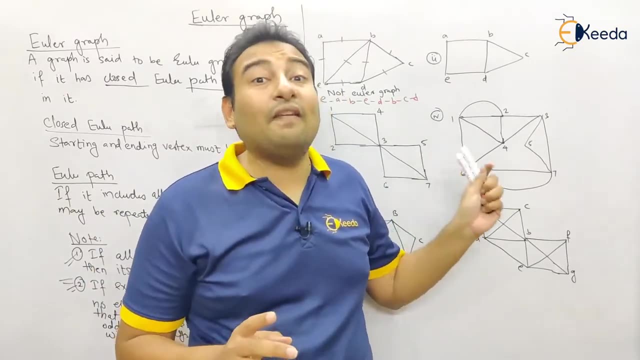 If we have three vertices with odd degree. first of all, it will not be a Euler graph, because the condition is all the vertices should have E1 degree as well, as there will be no Euler path, because Euler path exists only if two vertices with the odd degree. 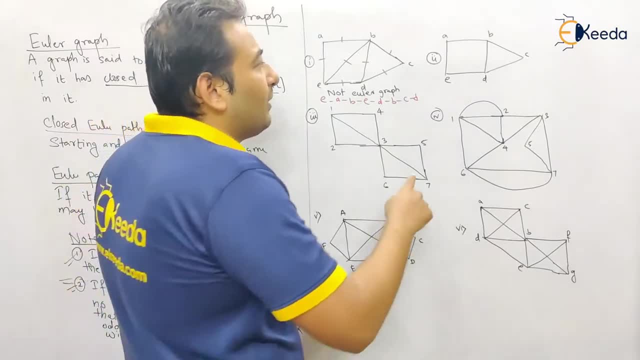 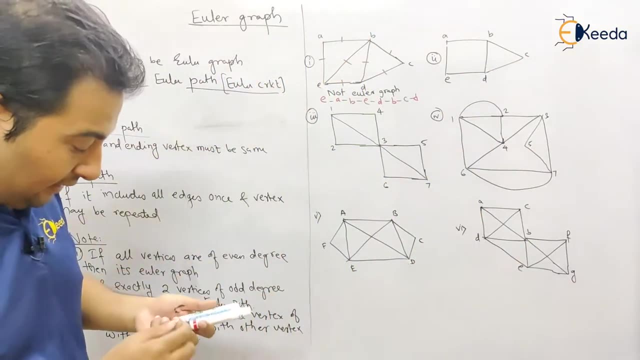 Is this clear? Let us move on. Let us discuss the next graph. Now let us check. This is E1.. This is E1.. This is odd, This is odd and this is E1.. So what do you mean by that? 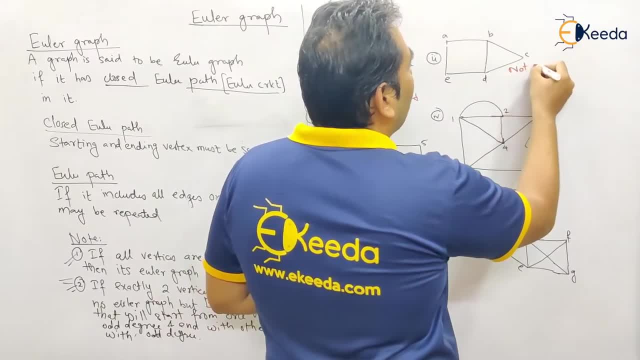 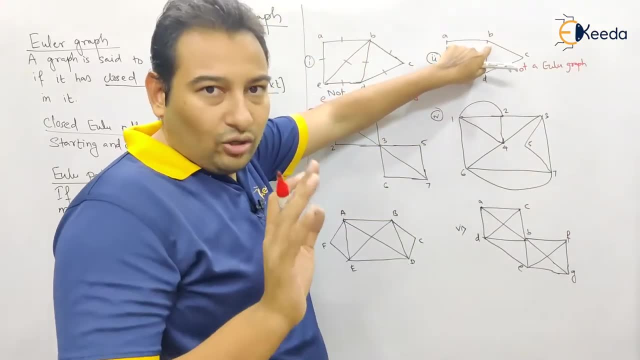 Since odd. so, first of all, not a Euler graph. Why not a Euler graph? Because there is a vertex with odd degree. not a Euler graph. Now let me check. Will there be a path? Euler path? This is odd. 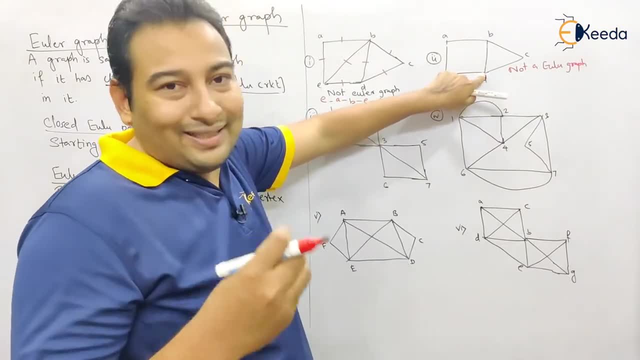 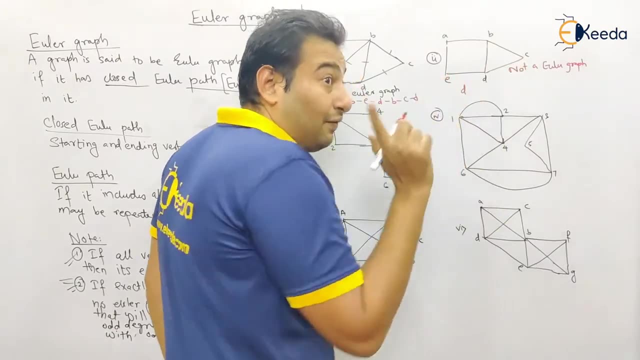 This is odd: Exactly two vertices of odd degree. That means there will be a Euler path that will start from one vertex with the odd degree. So I'm starting with D, You can start with B. also, You cannot start from E- One vertex with the odd degree- and should end at the other vertex. 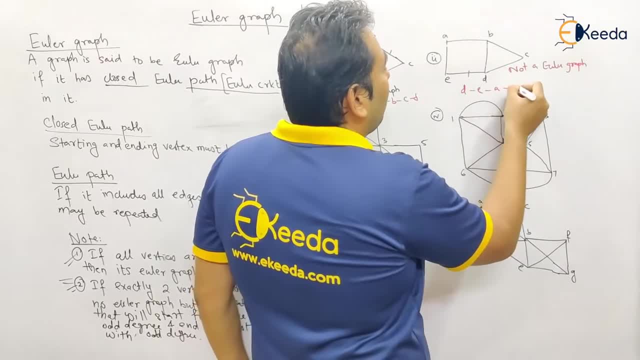 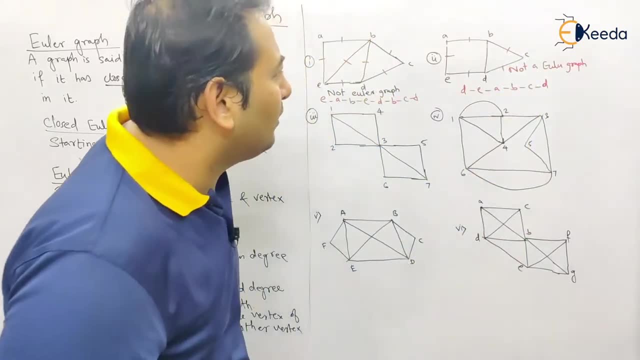 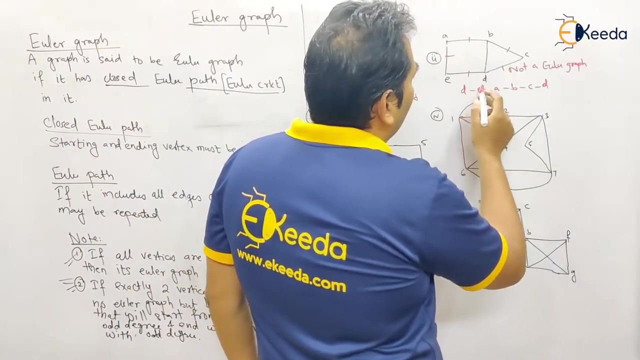 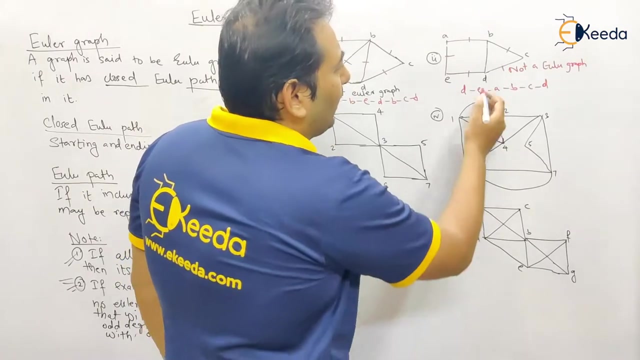 With the odd degree. So let me start: D, E, A, B, C and D. That's it, So very simple story. And from D, this edge is left, So we'll go to B. Now all the edges are traversed once. 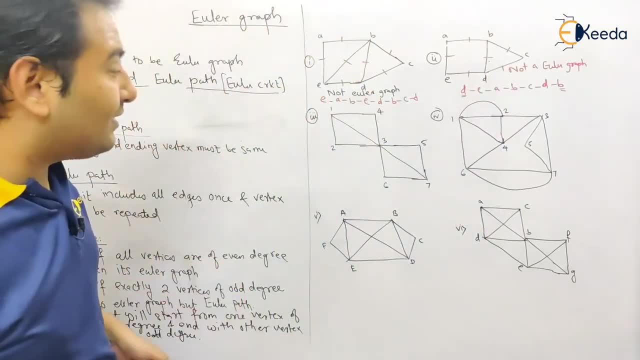 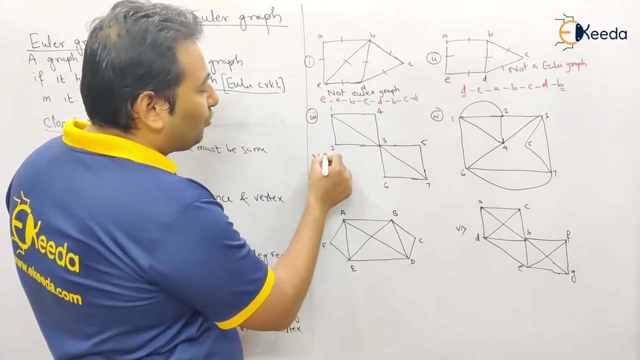 Starting point is D, ending point is B. Let's move on. Let us discuss the next graph. Again, if you check one vertex, this vertex with the odd degree, So obviously it will not a Euler graph, So obviously there will be not, will be a closed Euler path. 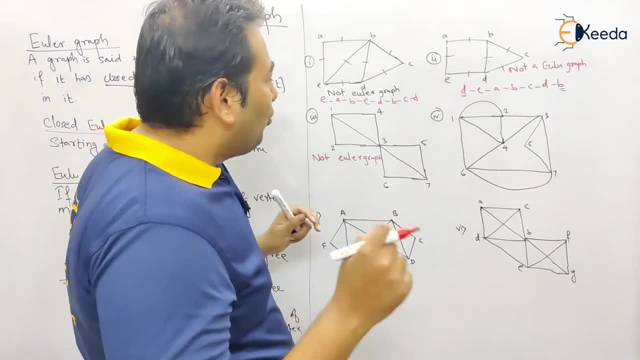 Still check. will there be a path when, if there are two vertices with the odd degree- See, this is odd degree. This is odd degree. This is E1.. This is E1.. 1, 2, 3, 4, 5, 6.. 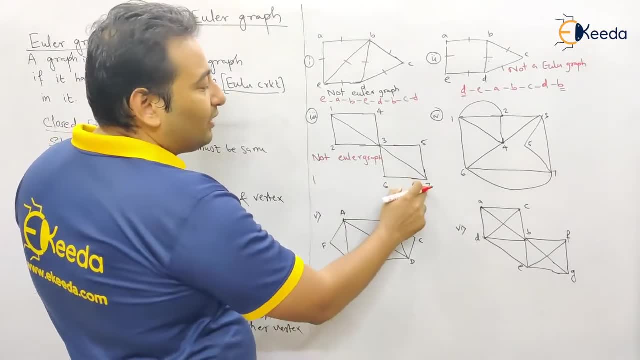 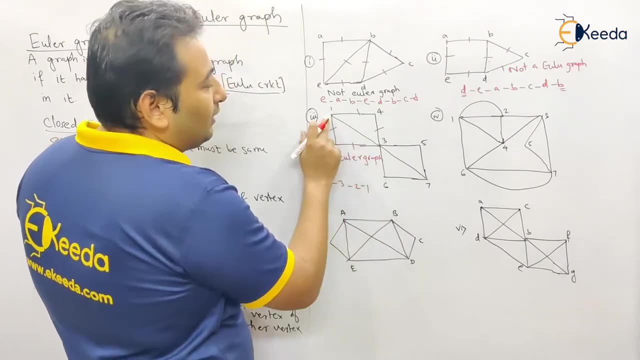 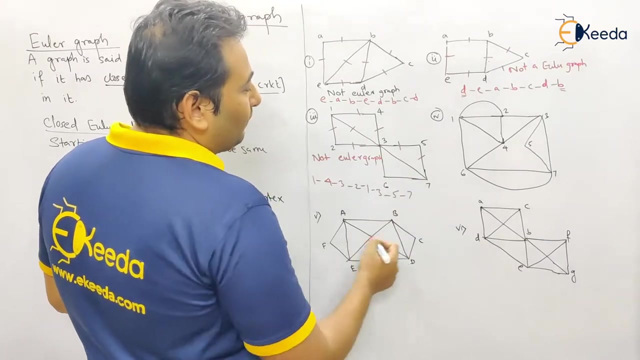 This is also E1.. That means there will be a Euler path: Start with 1 and end with 7.. So let me check 1, 4,, 3, 2 and back to 1,, then 3,, then 5,, then 7,, then 6,, then 3 and finally 7.. 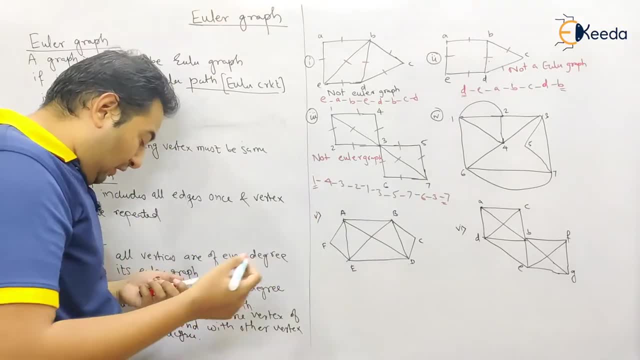 So see: started with 1, ended with 7.. Vertices may be repeated, No problem. Let us move on. Let us discuss the next graph. Let me check this particular graph: 1, 2,, 3, 4.. 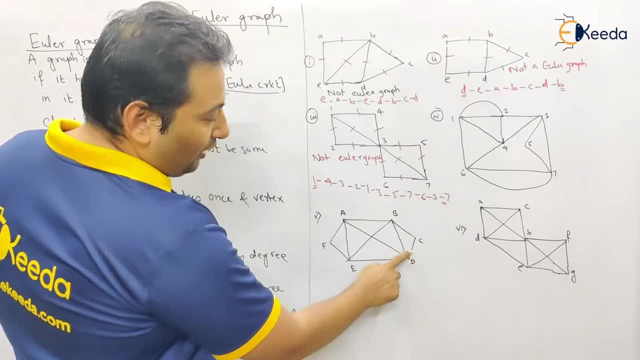 This is E1.. 1,, 2,, 3, 4.. This is also E1.. This is E1.. 1,, 2,, 3, 4.. This is E1.. 1,, 2,, 3, 4.. 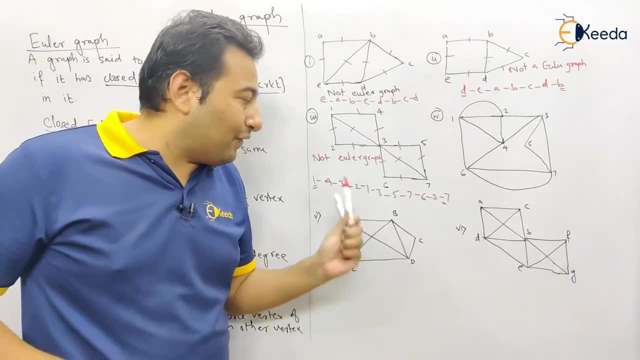 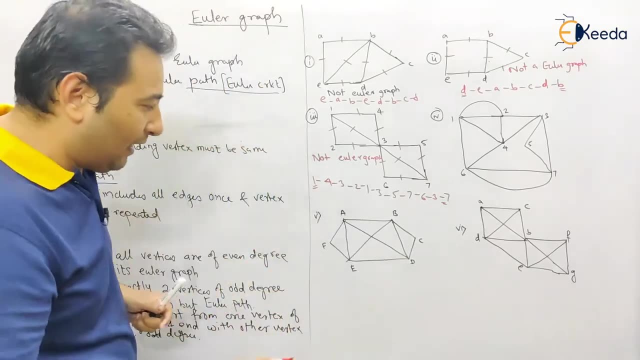 This is also E1.. This is also E1.. That means all the vertices have E1 degree. Therefore, it's what a Euler graph? That means there will be closed Euler path. So let us check that Euler path. So let me start with A. 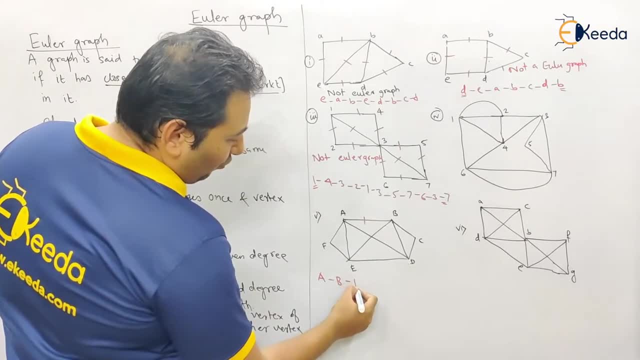 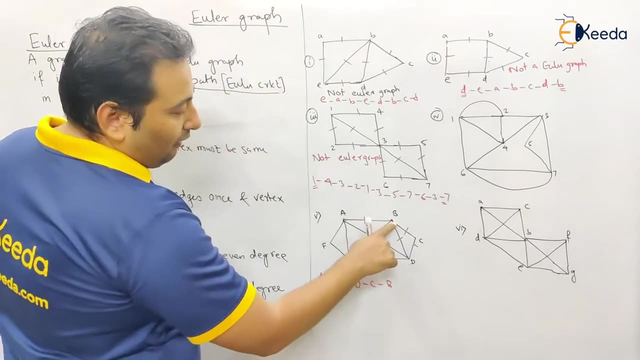 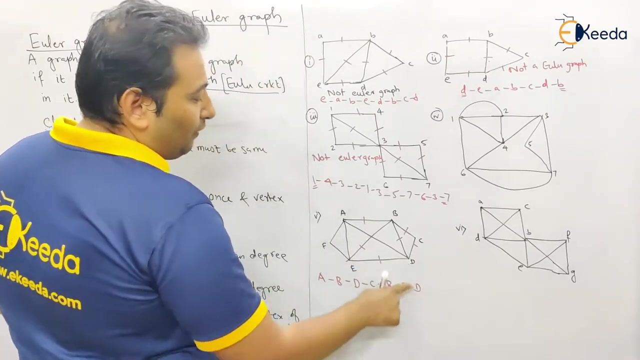 So from A you can go to B, From B you can go to D, From D you can go to C, From C you can go to again B, And from B you can go to E, From E you can go to D. 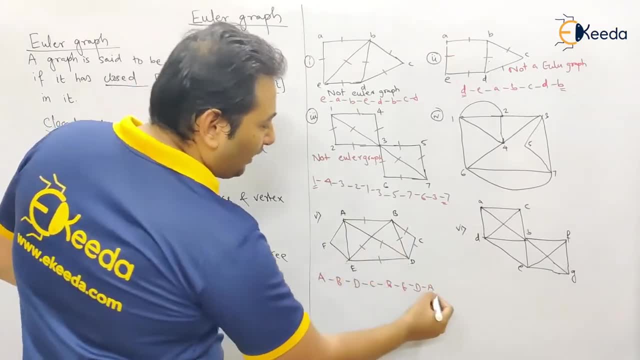 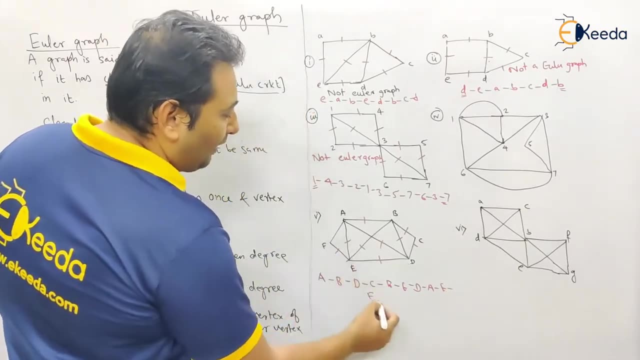 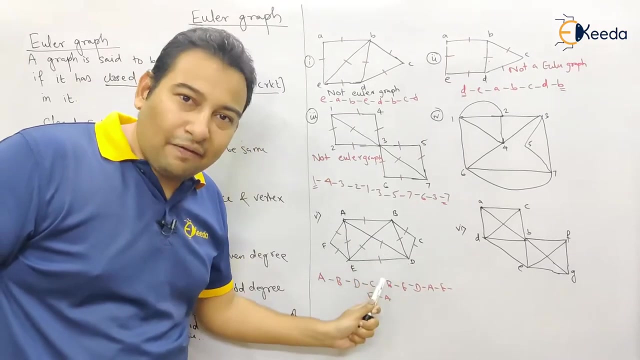 From D you can go to A, From A you can go to E, And from E you can go to F, From F you can go to A. See here, All the edges are visited once See. no edge left. 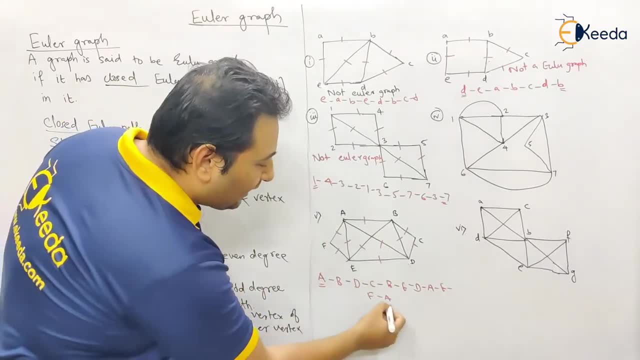 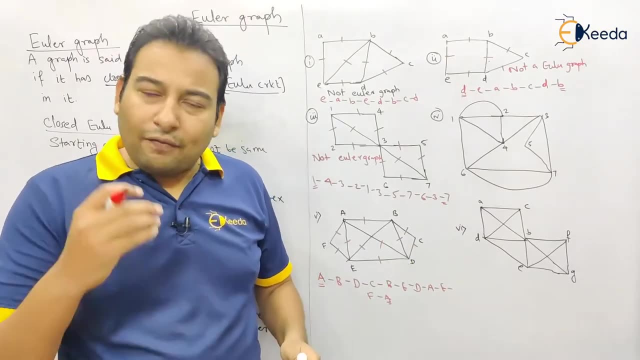 And they all are visited once, Since the starting and ending point is same. therefore it is a closed Euler path And obviously we identified the graph is Euler graph, So there must be a Euler path, closed Euler path, So the starting and ending point is same. 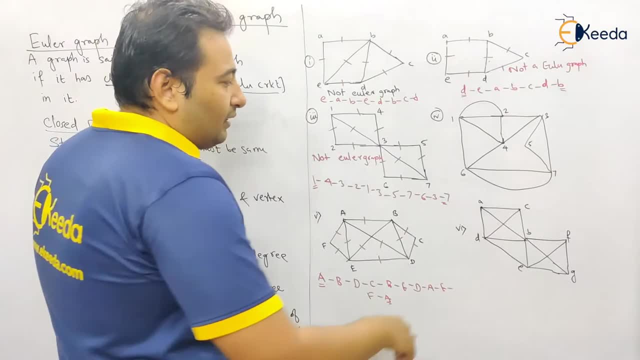 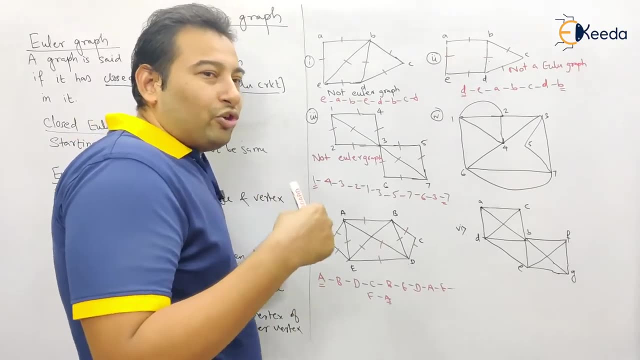 Is this clear? Let us move on. Let us discuss the next example. So this is my next example. It's degrees 3.. It's not a Euler graph. Now let me check: Is there any possibility of Euler path? There may be a possibility of Euler path if there are exactly two vertices with this. 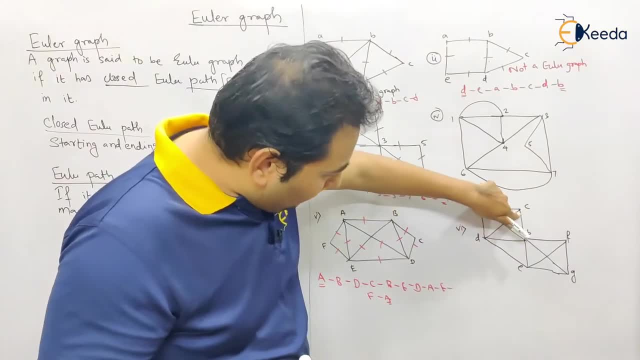 This is with odd degree. This is with odd degree. This is with odd degree 1,, 2,, 3, 4.. This is even 1, 2,, 3,, 4,, 5, 6.. 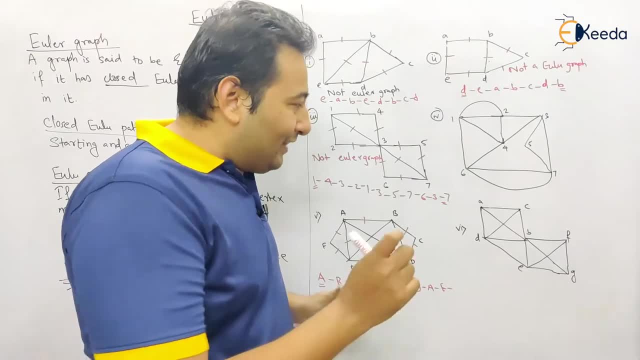 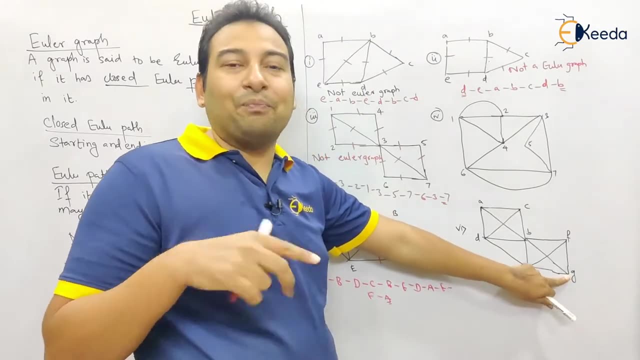 This is also. even This is odd. Now, in this particular graph, there are three vertices with odd degree. There are actually four vertices. So it doesn't matter to me, I just want to check. See. first of all, it's not a Euler graph. 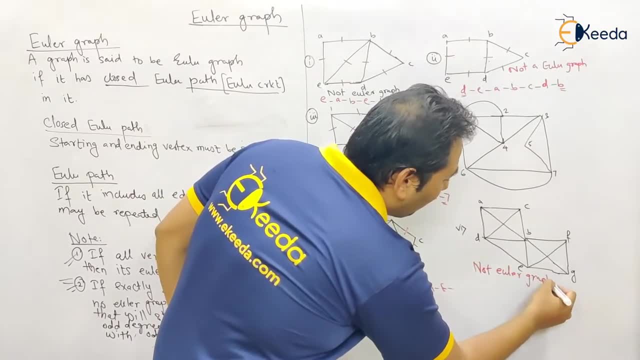 I hope this is clear. Why not? It's a Euler graph, because there are vertices with the odd degree. Now my aim is to check whether exactly two are odd degree or not. This is odd. This is odd. This is odd. 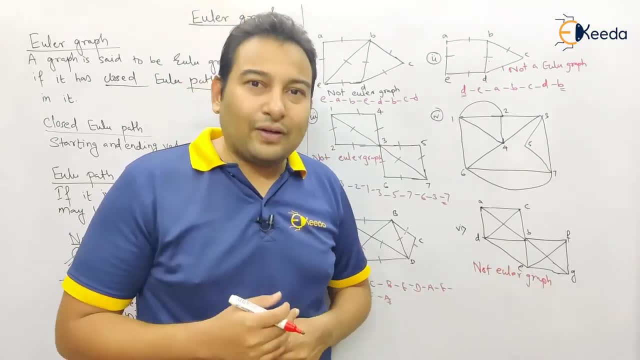 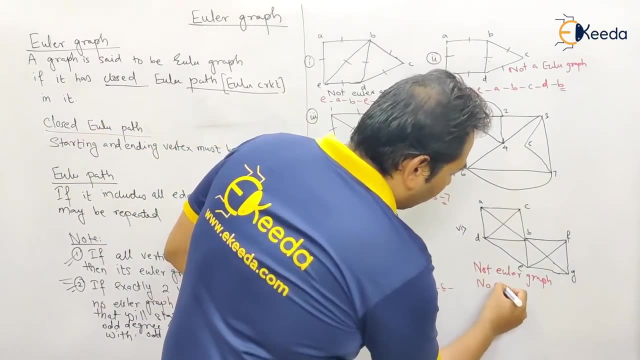 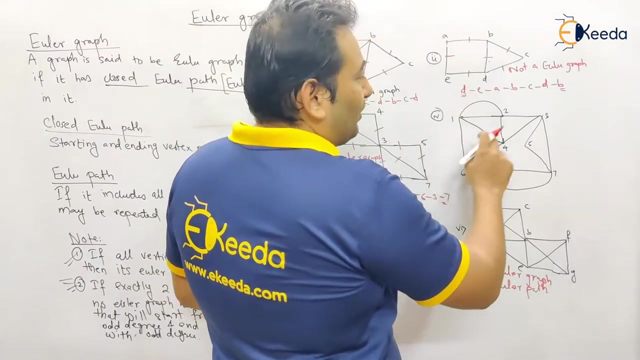 Story over. No need to check further because we found out three vertices with the odd degree. That means no Euler graph, no Euler path. Let us discuss the last example: 1, 2, 3, 4.. This is even. 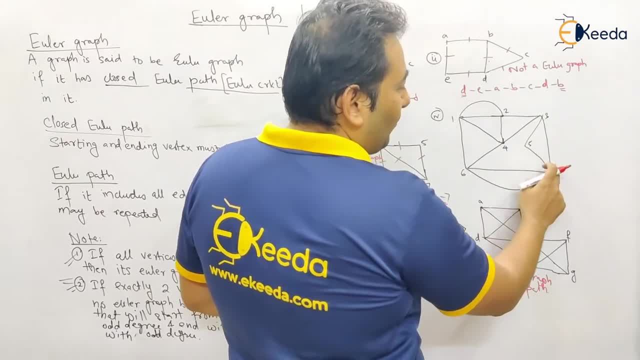 1,, 2,, 3, 4, even 1, 2,, 3, 4.. This is also even, This is even 1, 2,, 3,, 4, even This is also even. 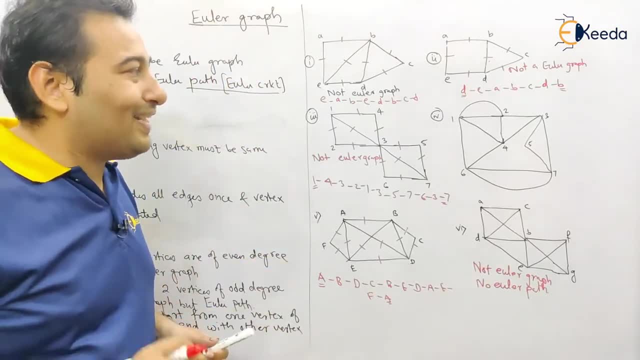 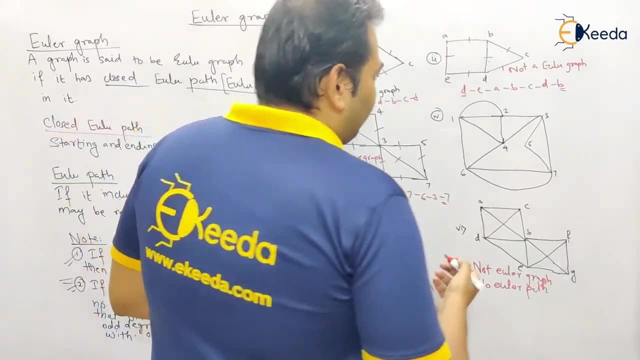 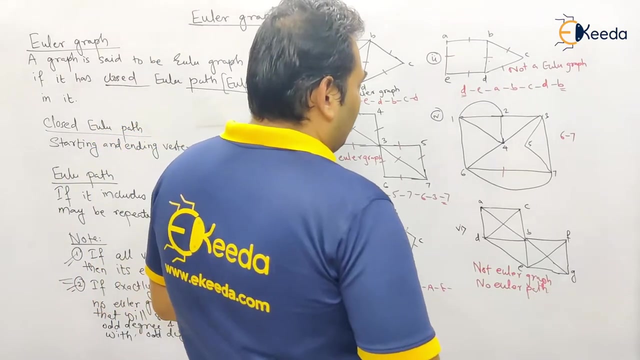 This is also even. That means all the vertices are of even degree. Therefore it's a Euler graph. Since it is a Euler graph, there must be a closed Euler path. So let us start 6, 7.. See from 6 to 7.. 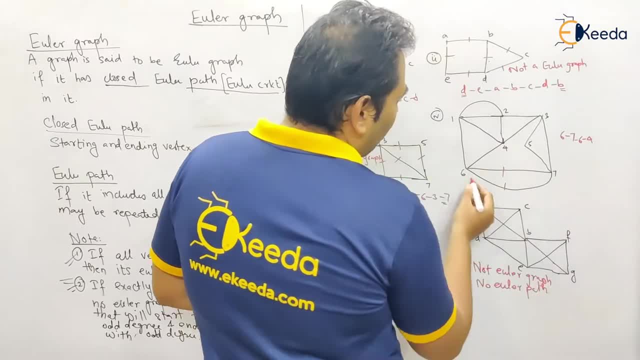 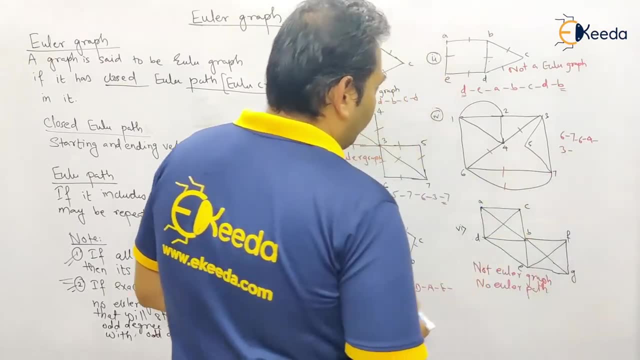 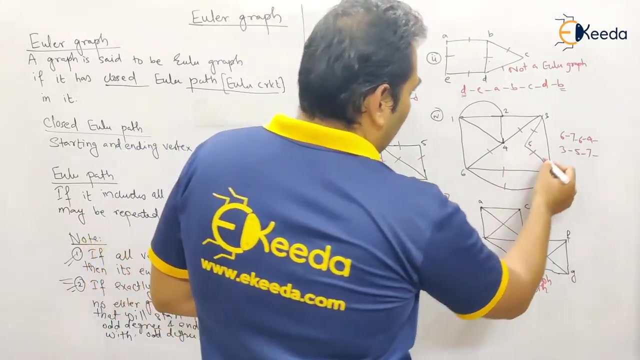 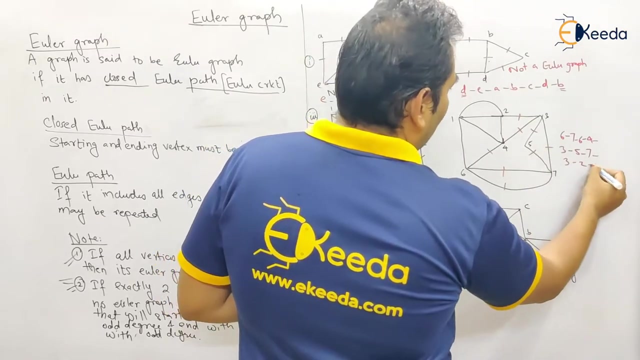 From 7 to 6.. From 6 to 4.. From 4 to 3.. From 3 to 5.. 5 to 7.. From 7 to 3.. From 3 to 2.. From 2 to 1.. 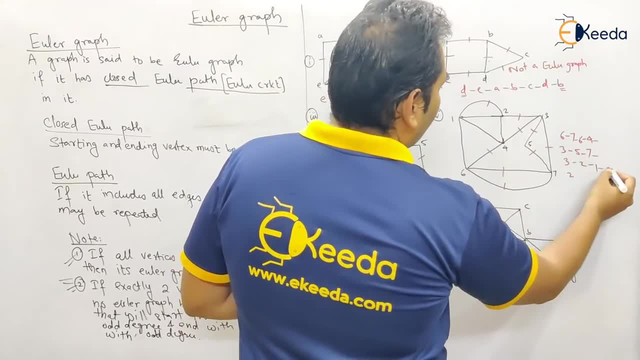 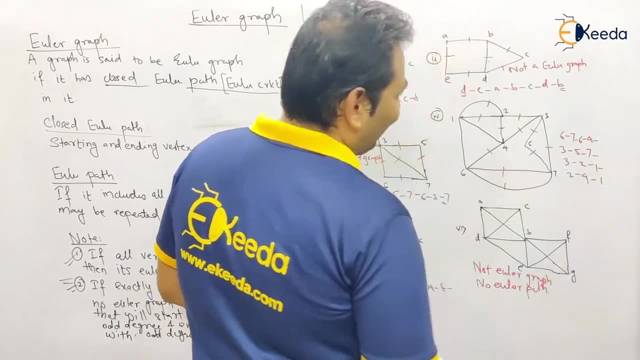 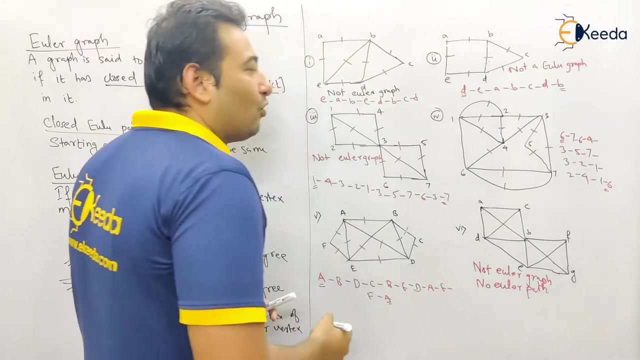 From 1 to 2.. From 2 to 4.. From 4 to 1. And from 1 to 6.. See, the starting and ending point is same And all the edges are the same, Because Euler is not restricted on the vertices. 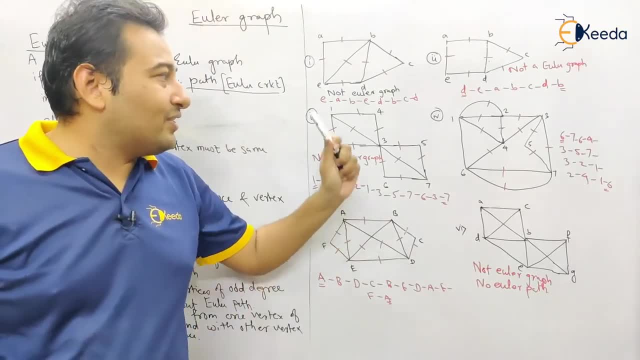 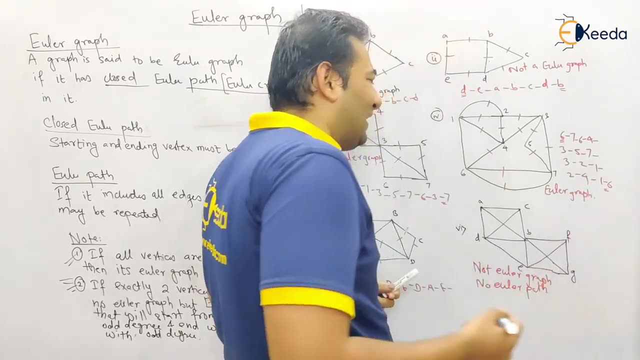 All the vertices are traversed once, No restriction on vertices. So this is your Euler graph. Is this clear? So I think this much practice is enough. Now you can pick any textbook or you can refer, You can go to internet and you can pick the question. 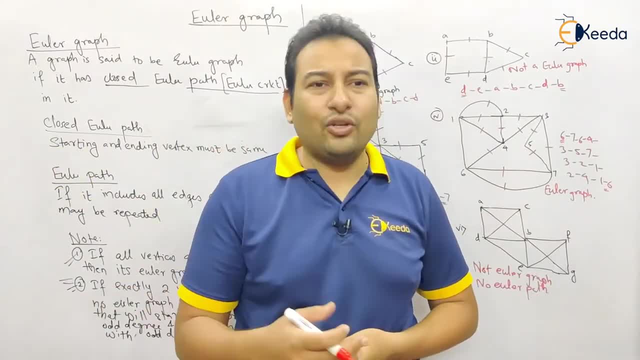 And you can verify whether it's a Euler graph or not. How to remember? See, there is a concept: Each and every h must be visited once, Since it is Euler. How to remember Euler? e, h, e. So that is what I wanted for you. 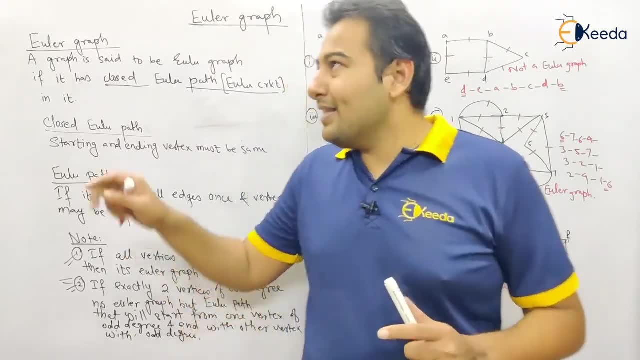 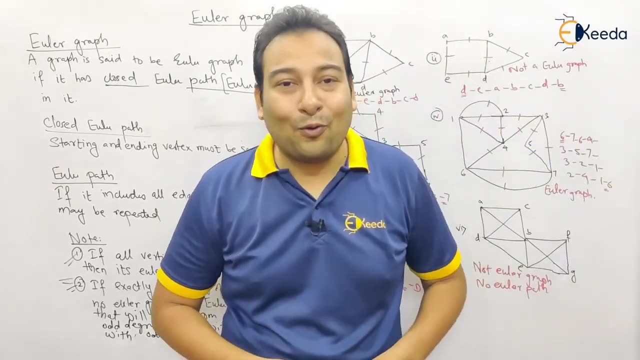 So this is an example for you. So here you can see how to remember Each and every h must be visited once, Since it is Euler. how to remember Euler: e, h, e. So that is what I wanted for you about Euler graph. Hope you understood. Thank you for watching this video. Take care.